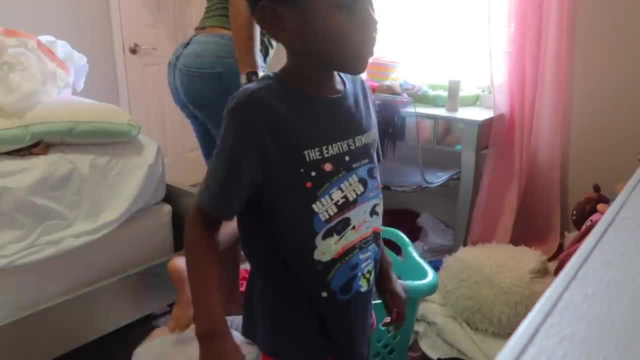 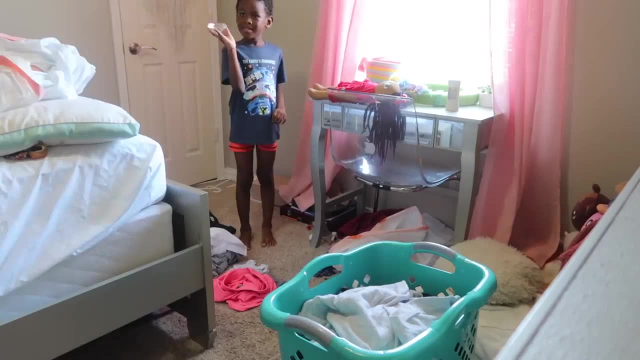 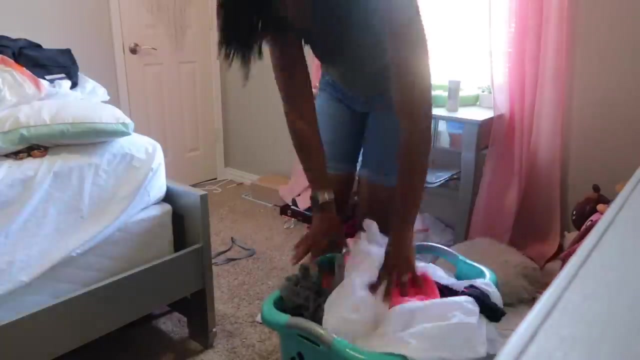 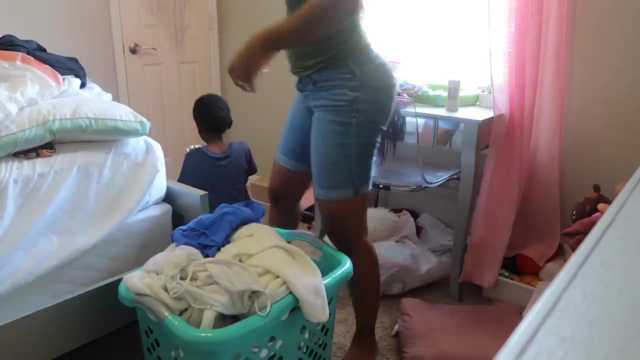 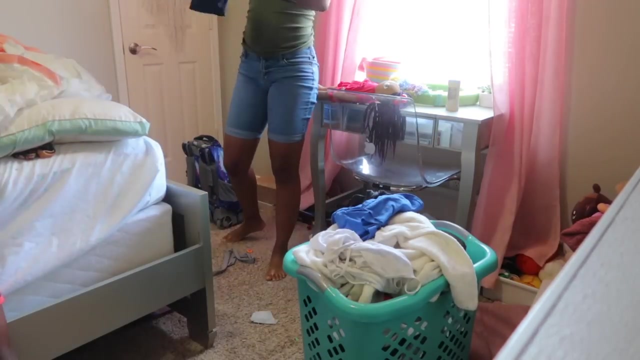 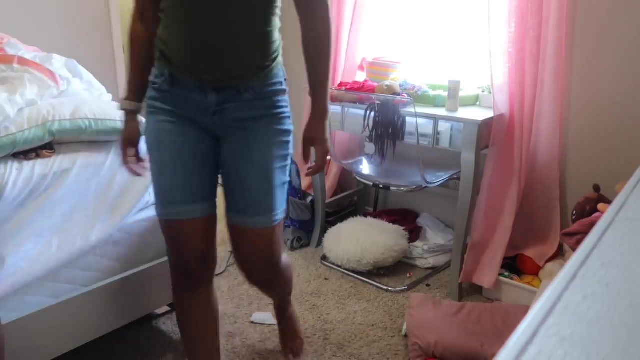 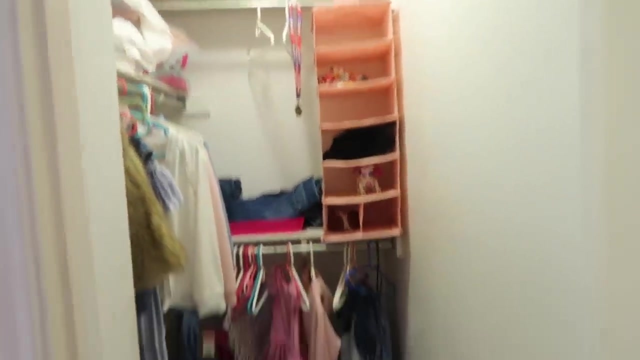 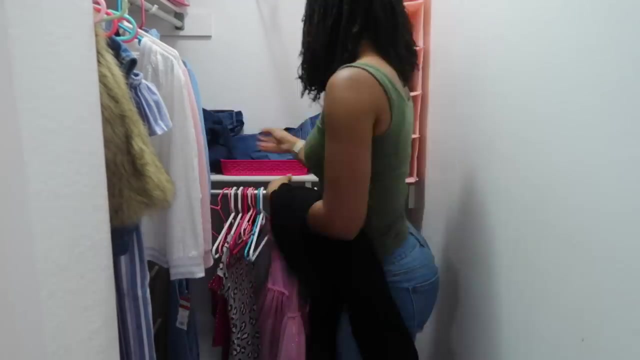 yeah, as you guys can see how bad her room really is, I wanted to let you know that it does go from bad to worse. I had to show you her closet now. I will admit I have been avoiding her room for a while because it's just so much work and it is really hard for her to maintain. I was the same way as. 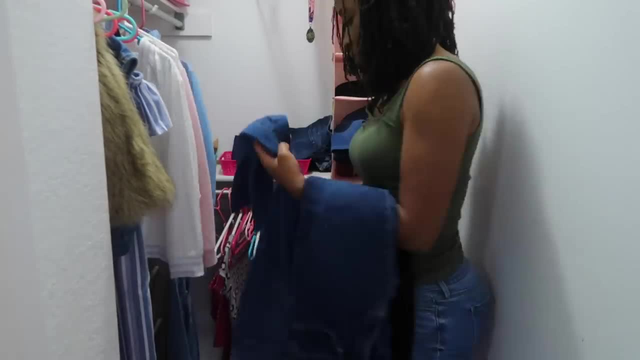 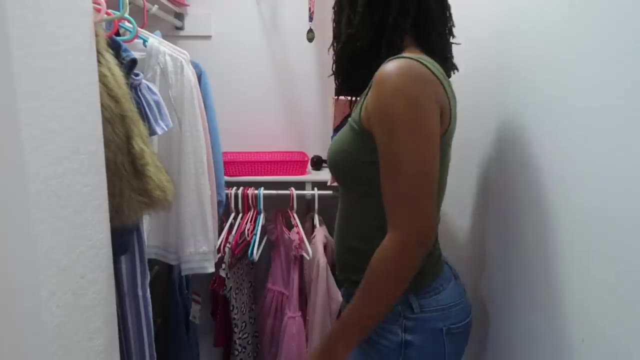 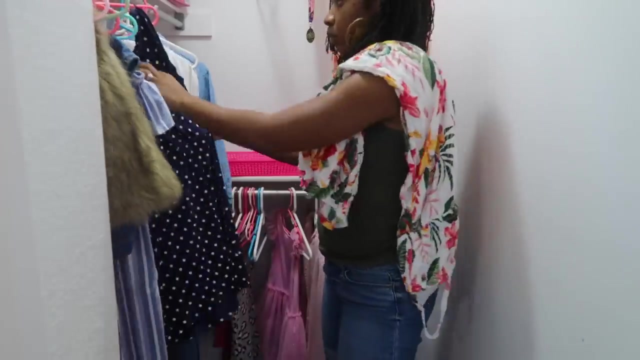 at her age. so I do understand, but it you know it's annoying and I don't want to do it that often, I don't. it just gets out of control. so it was time for me to step in and assist and get everything back in order so that we could function and try to keep up with it together. I'll admit I was a bit 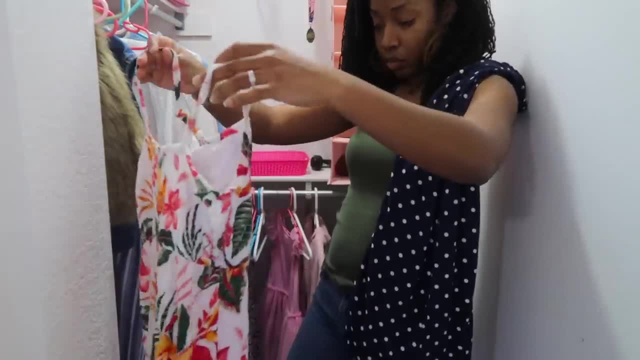 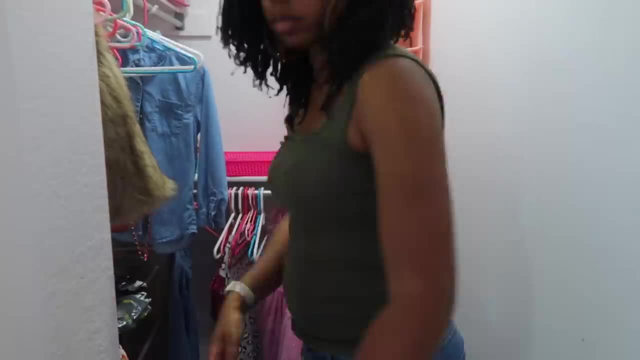 overwhelmed, but I just decided to take everything out. it wasn't my original plan to have to do all of these things, but I decided to just take everything out of the closet completely. you'll see that in a moment. but I decided to just take everything out of the closet completely and I 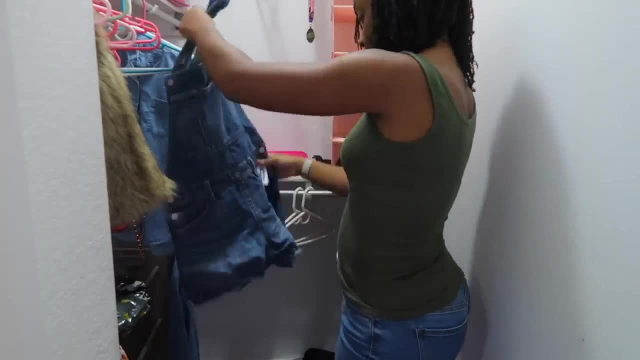 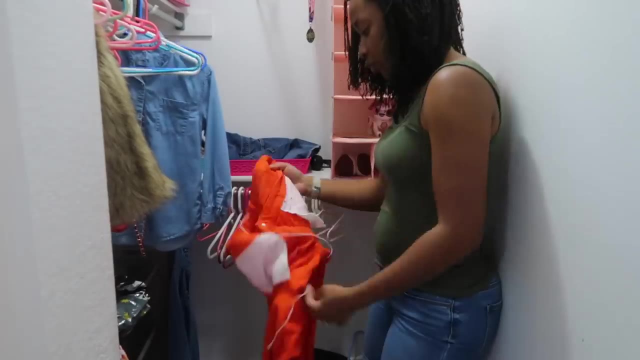 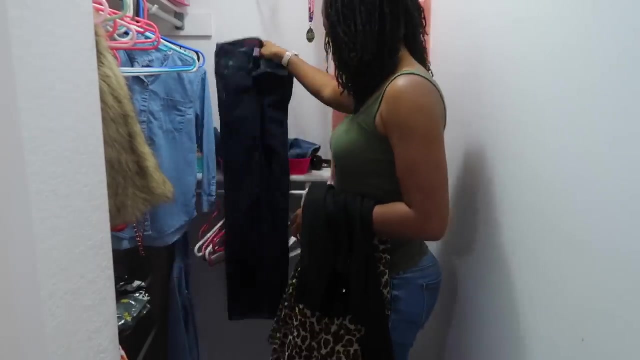 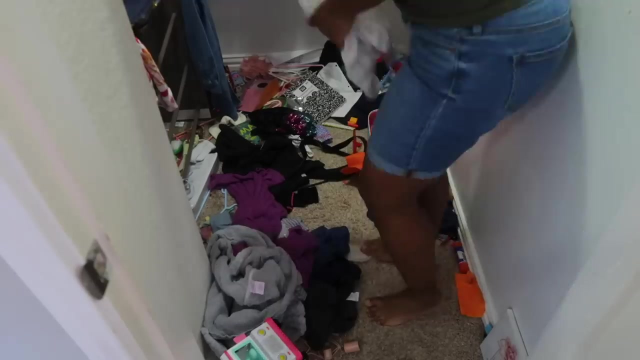 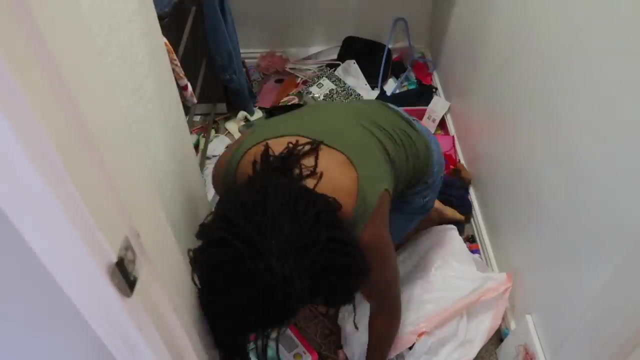 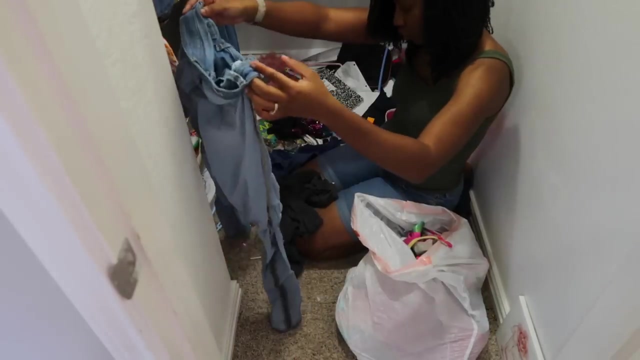 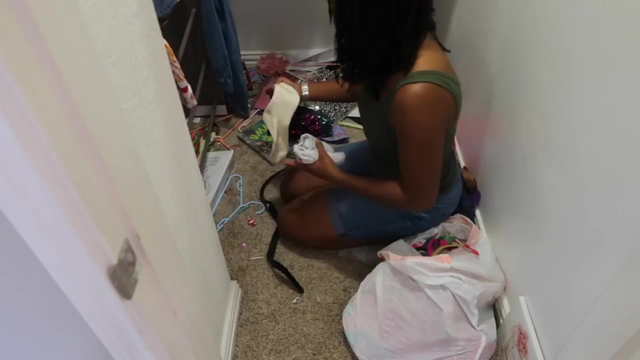 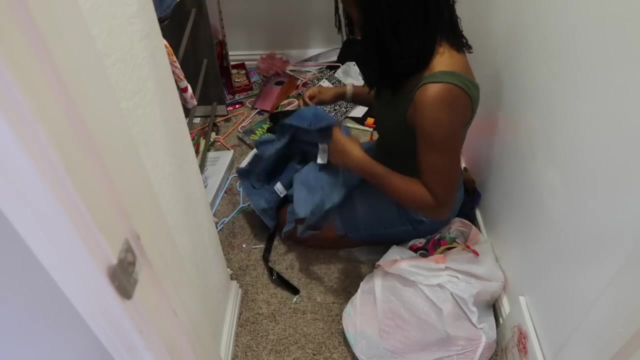 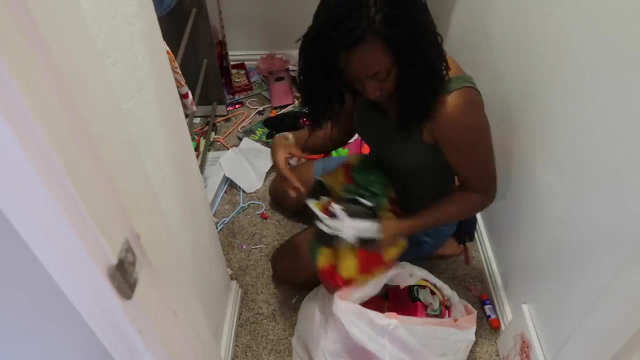 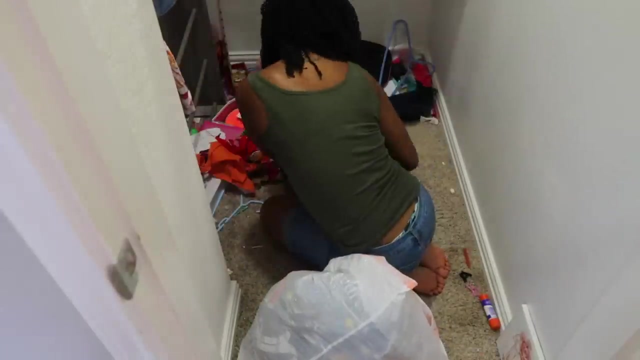 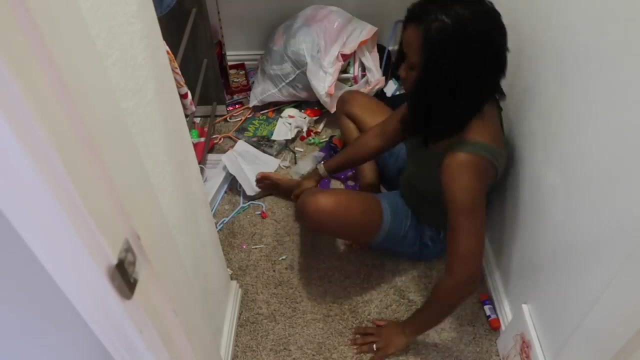 decided to take everything out and just start from scratch, because there was just no way to organize this chaos. otherwise, I forget that we're done, that you're back with your girlfriend now for a minute. I'm back where we started. in that hallway we couldn't keep our hands away from each. 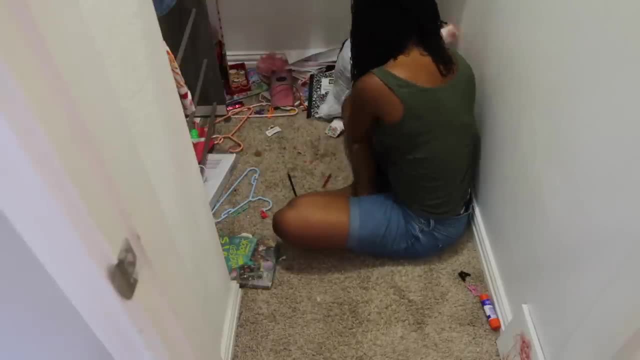 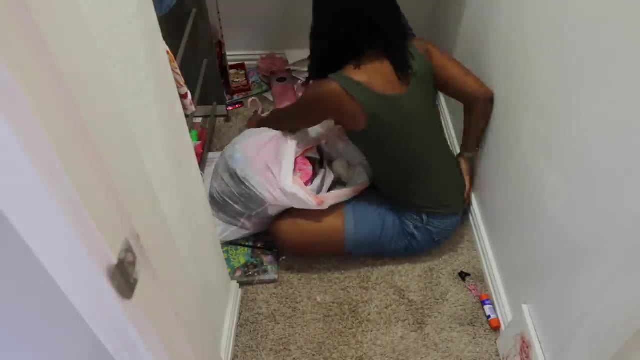 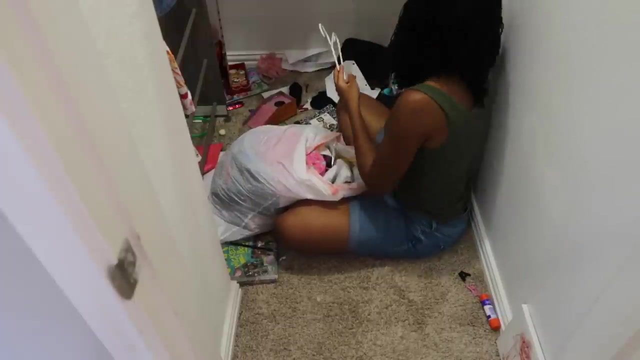 other. so I was trying to be reasonable and go through everything so I could try to keep the things that I know she would like, or maybe I would ask. and then I realized, like this is not, this is pointless. this is why we always end up in this situation, because she collects the, she just 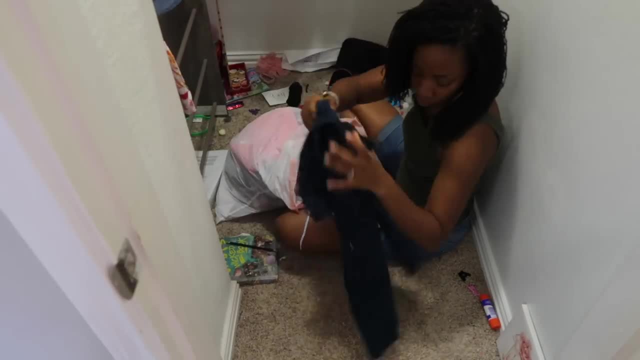 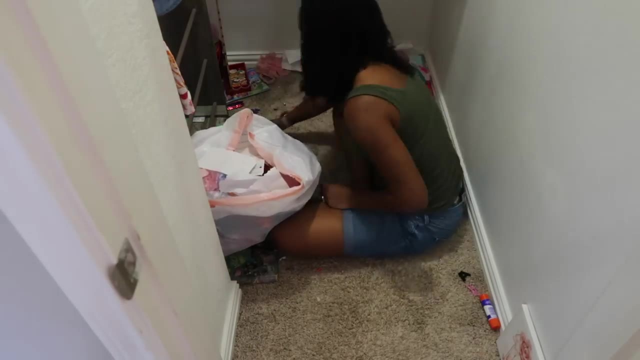 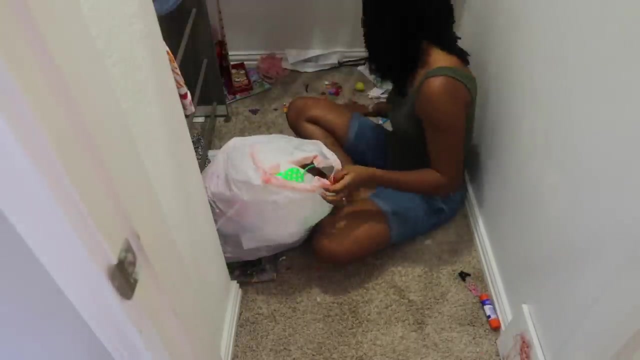 collects everything. there's just so much junk and things on her closet floor. at one point we she wasn't even putting clothes in the closet because it was just so much junk in here. so I am going to throw everything away, everything, everything that's on the floor, all the little toys, because 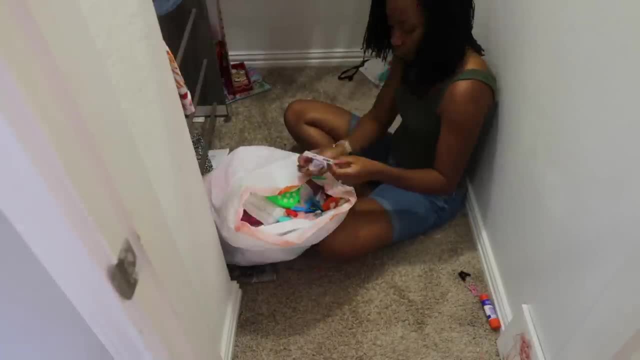 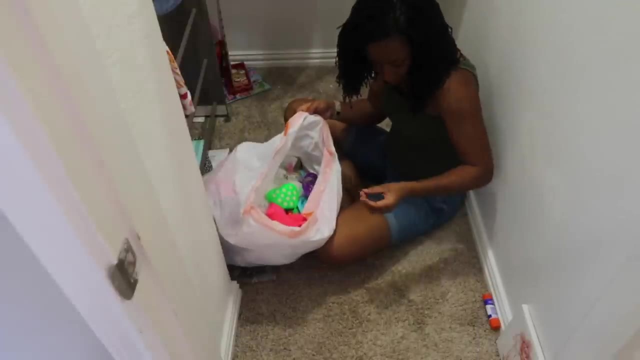 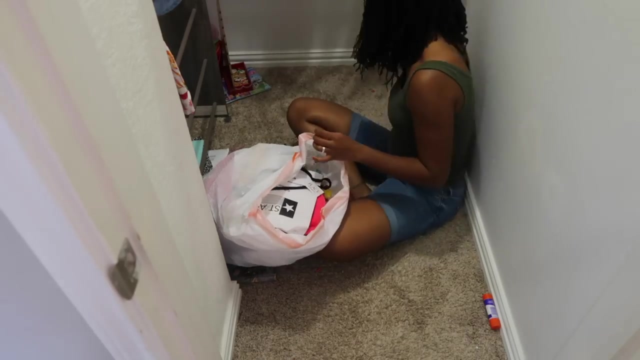 she honestly does not play with anything of these things anymore. she's 12 years old. she still plays with little toys, but nothing that was in this closet. she was not going in that closet for anything- not clothes, nothing- because it was a mess, so I am going to clean it out completely. you'll see that at the end of this video, so that 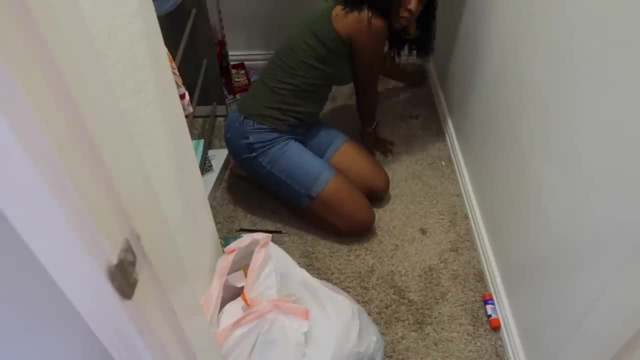 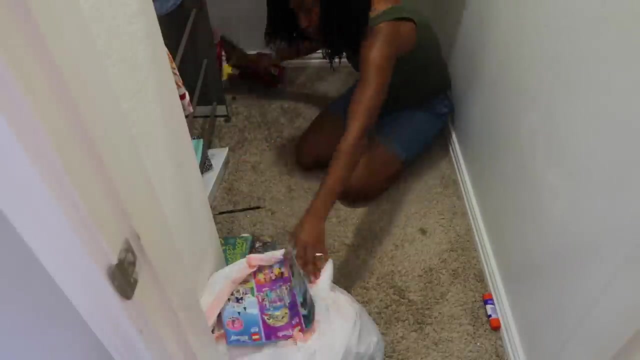 it's actually a functional closet. that was another reason why she had such an issue with clothes all around her room, because she couldn't utilize her closet because of all the junk that was in the closet, and I mean it's but so much clothes she can fit in her dresser, so it would just end up on. 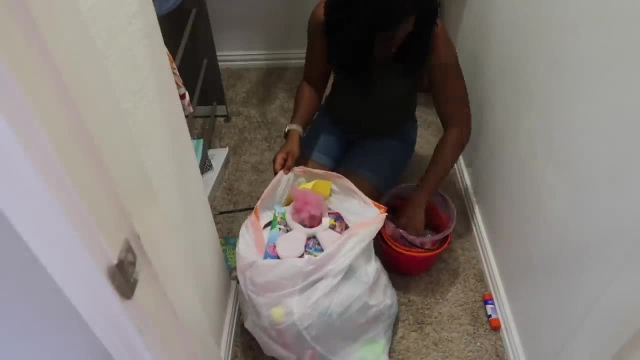 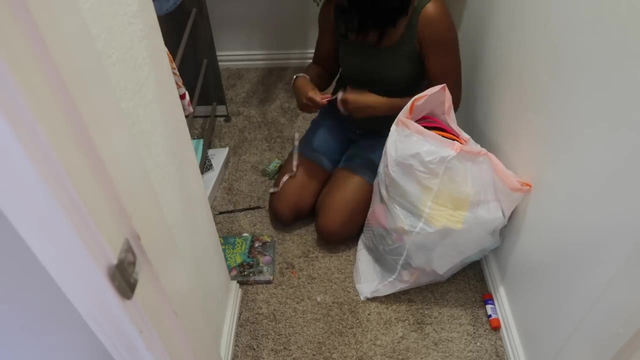 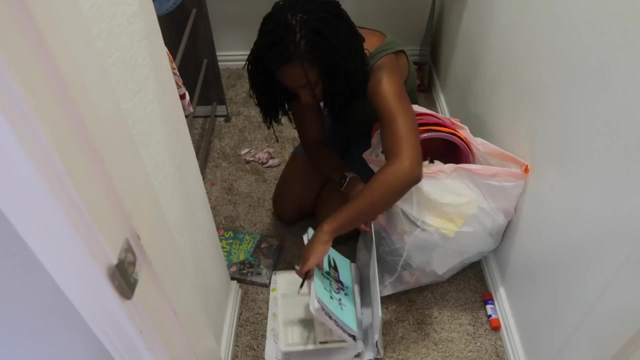 her bedroom floor. so, yeah, lots of problems we're solving by just cleaning out this closet. now I always pick you up and let you down. we're spinning around, losing our minds and if we do and if we don't, and if we give you what we want, 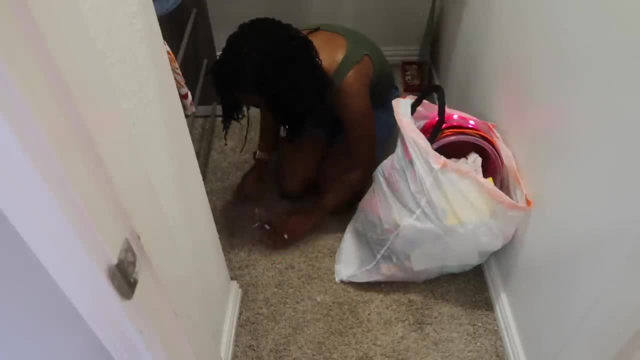 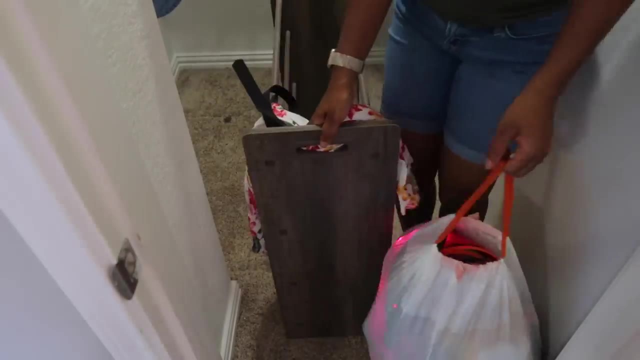 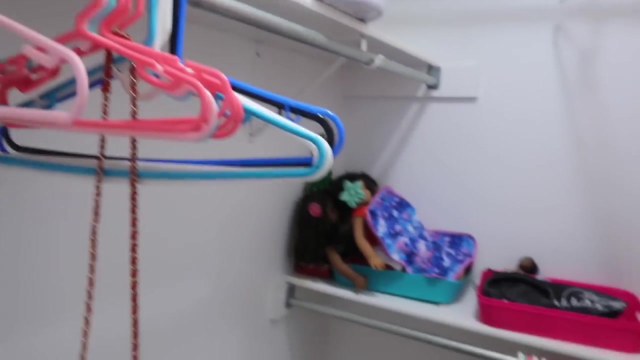 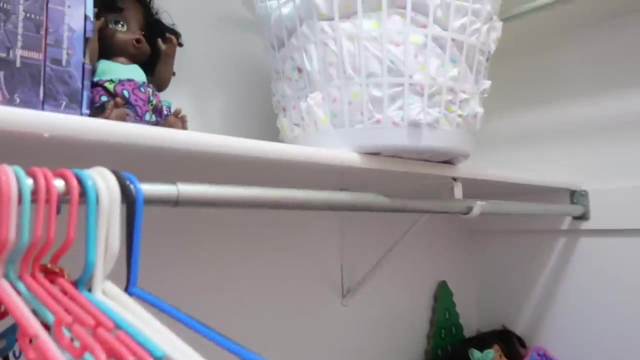 to walk. so here's what her closet looks like, with all the junk and clothes out. I did take that toy rack out and we are now using it as a shoe rack, since she doesn't use the toy bins anymore. but pretty much everything is cleared out. I do keep that basket up there on the shelf with extra. 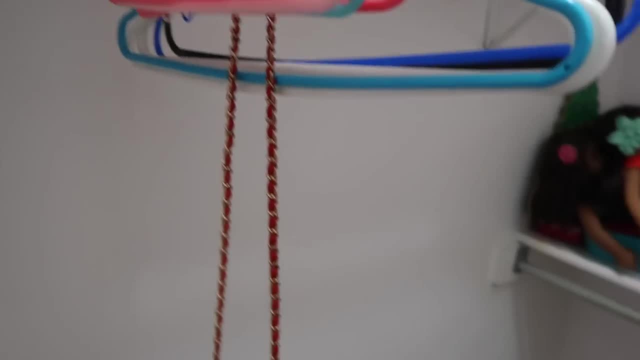 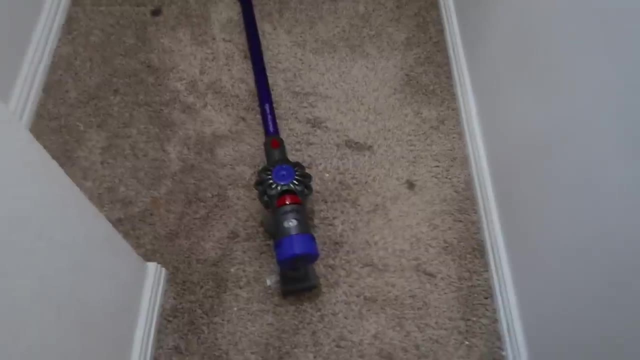 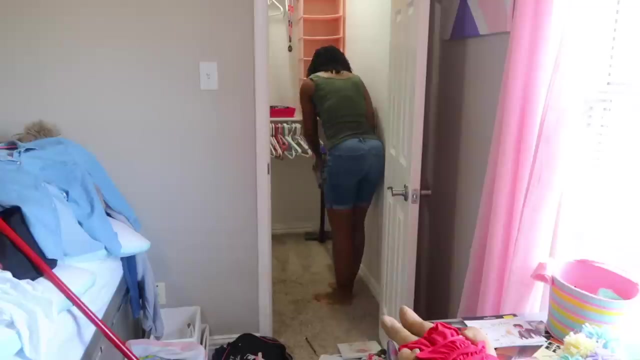 pairs of sheets for her, because, again, if you're new here, we don't have a linen closet in our house, so everyone just keeps their sheets in a basket in their closet. if you are not with me, hey, do you read me? go back back to where we came from. 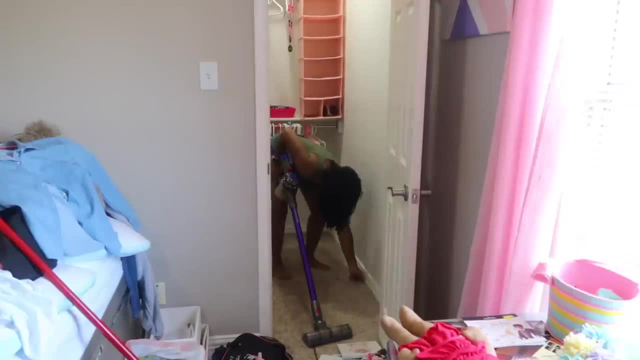 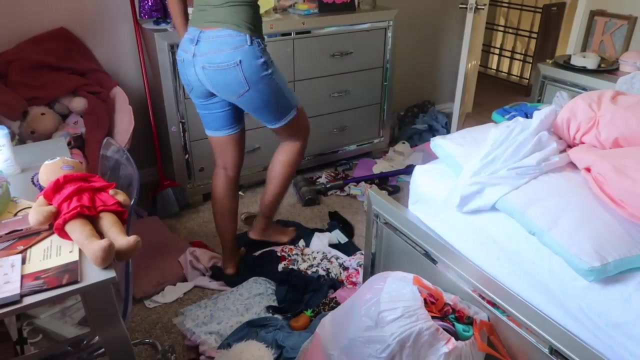 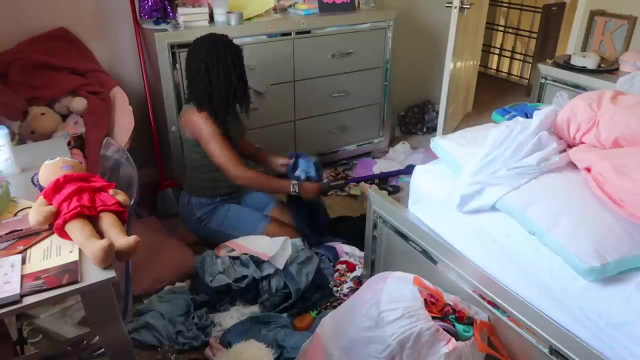 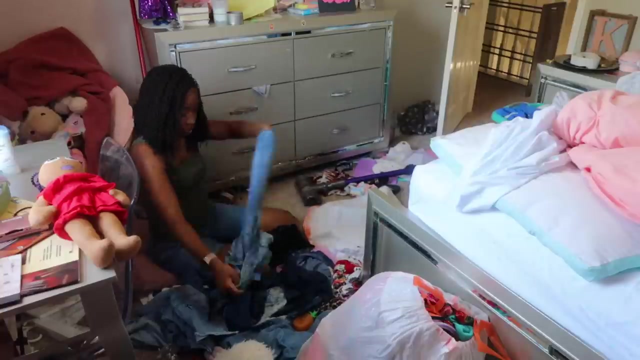 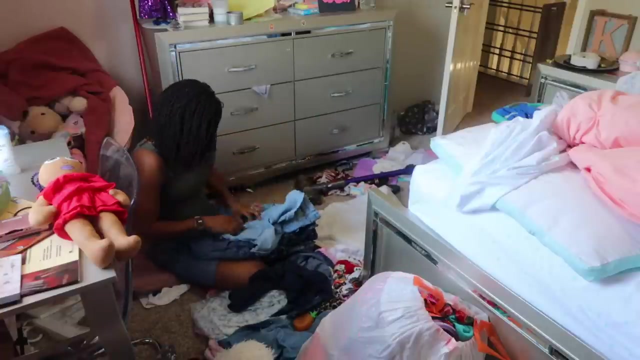 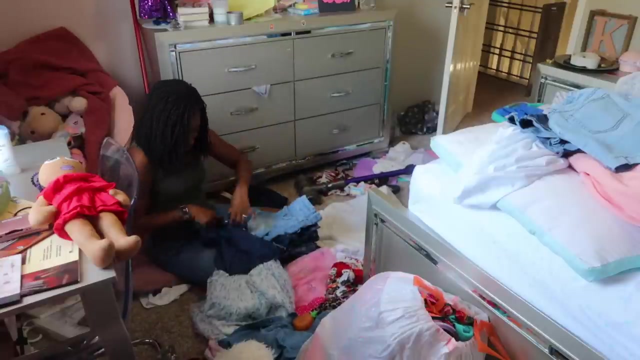 if my hands are empty? hey, do you read me? go back to where we came from. if my hands are empty, I don't wanna go alone. Go back If you wanna with me. I don't wanna go back If you wanna with me. Your intentions are good. I walk back to my history. 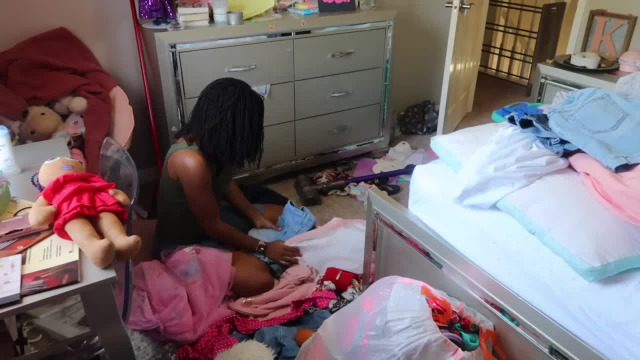 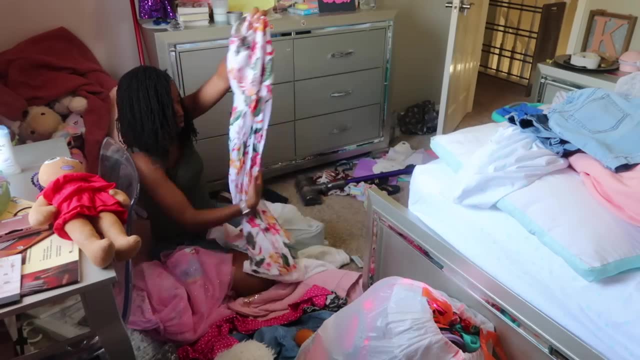 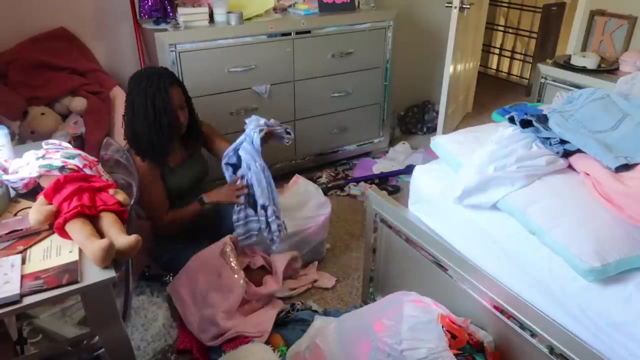 Into my own neighborhood Lying for you, lying for you, Oh, but I can't get back. What can I do? what can I do When your dream is gone? I don't wanna go back back. Don't wanna go back If you wanna with me. 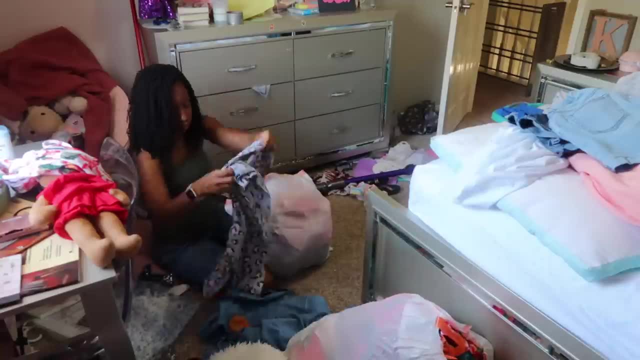 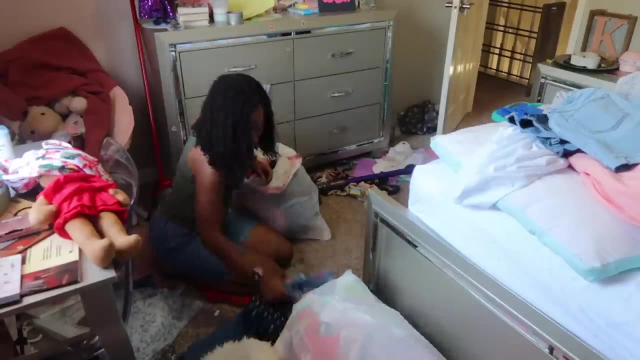 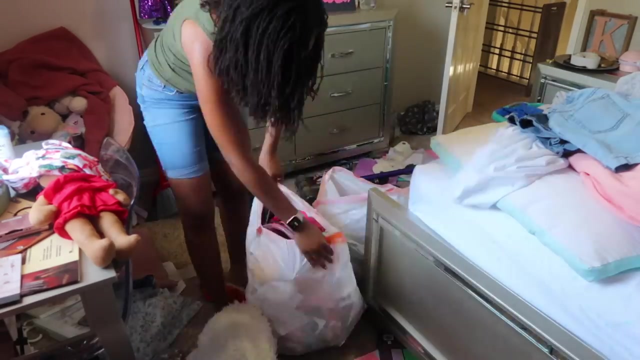 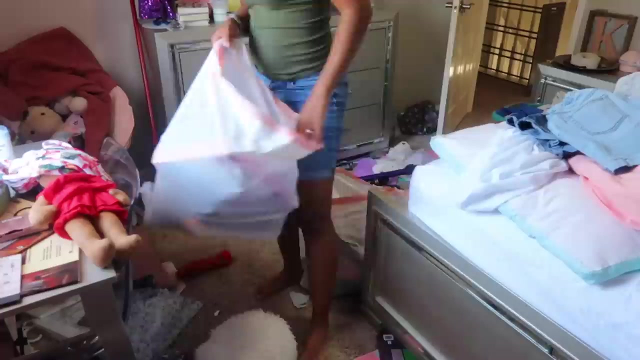 Baby, Baby, baby, go back back To where we came from. If my hands are empty, Hey, baby baby, go back. I don't wanna go alone. Go back. If you wanna with me, I don't wanna go back. So right here is when I realized: 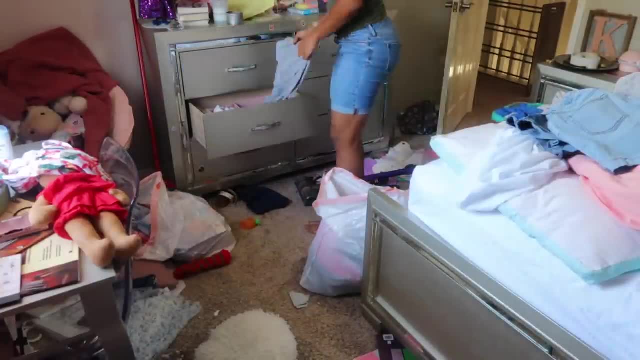 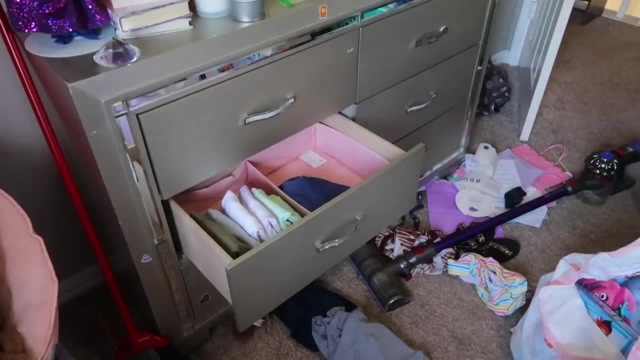 I was in a little like I was in over my head With this mess in here, But I was determined to get it done. I was definitely looking around the room like I should just throw the whole room away, But I get through it. 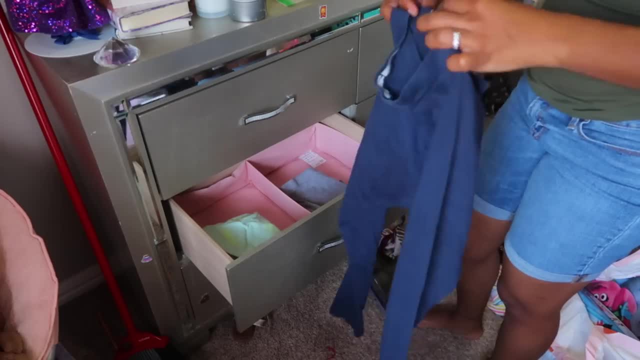 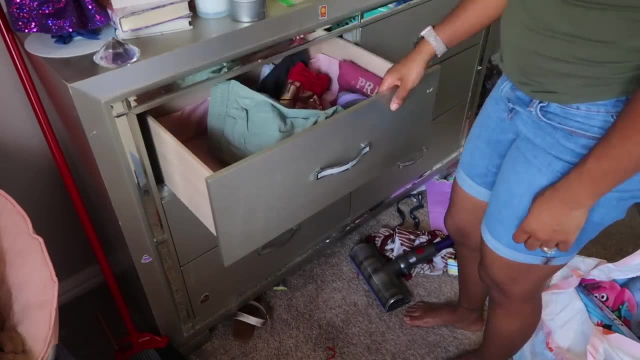 Now this is the part that frustrates me the most, because I organized her drawers in a way to make it very easy for her to keep up with and maintain, But never Like she just struggles with that. Like that top drawer should be for long-sleeved shirts. 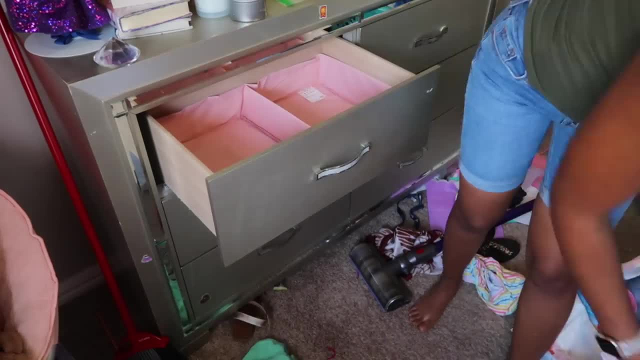 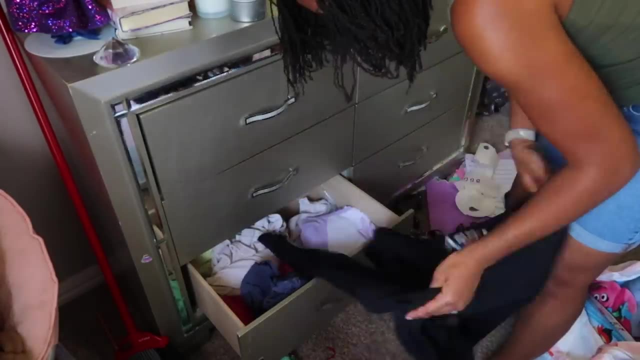 And there I pulled out three pairs of shorts out of that drawer. It's long-sleeved shirts, then short-sleeved shirts. We have like long pants, like leggings, then shorts, And the two bottom drawers are for like. 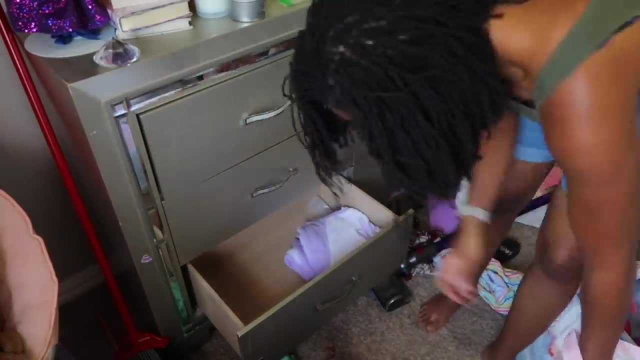 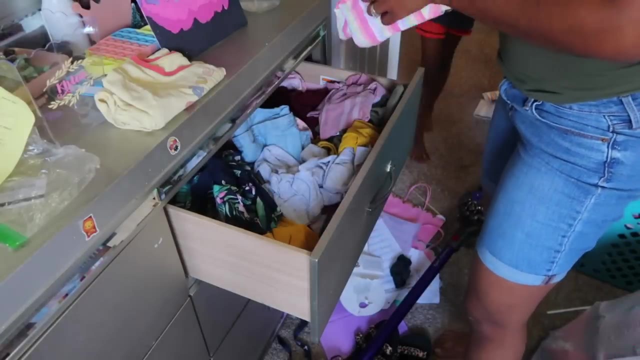 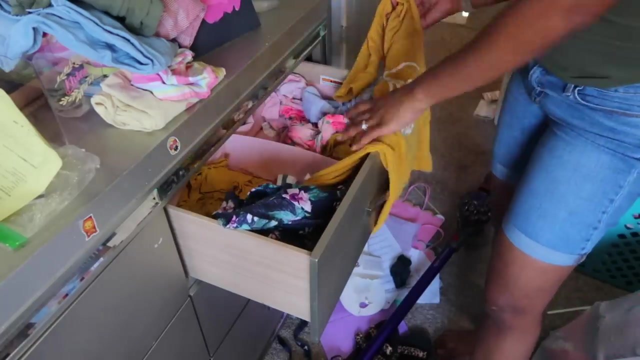 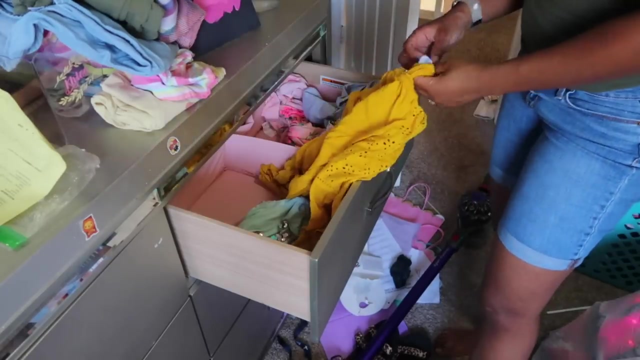 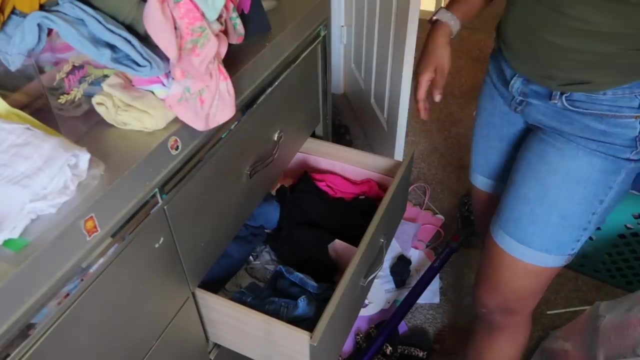 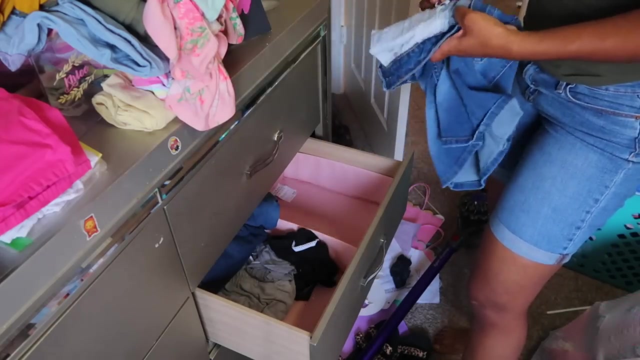 pajamas and miscellaneous things, house clothes and things like that. Very simple, Yet apparently very complicated. So again, I'm taking everything out so I can refold and organize. I'm just sorting through it because I do not want to. 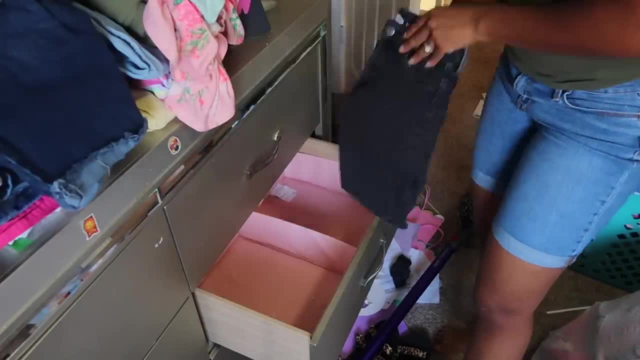 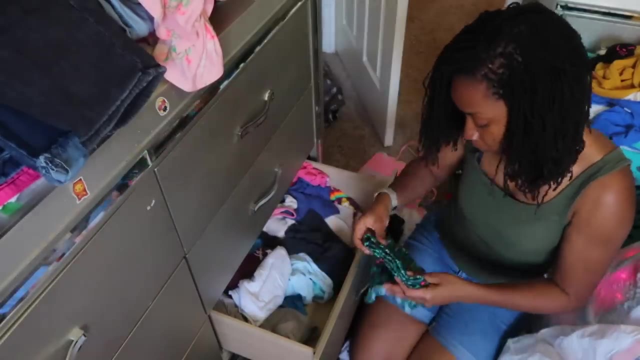 put anything back in that is too small or she has not worn since I bought it. if it's something that she's not wearing, I also want to get rid of it as well. so I'm just sorting through everything so I can get rid of things as I go. 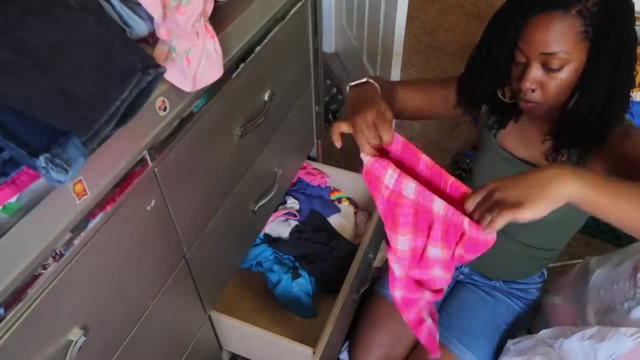 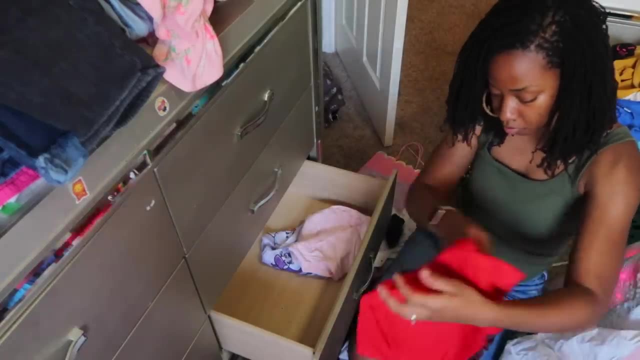 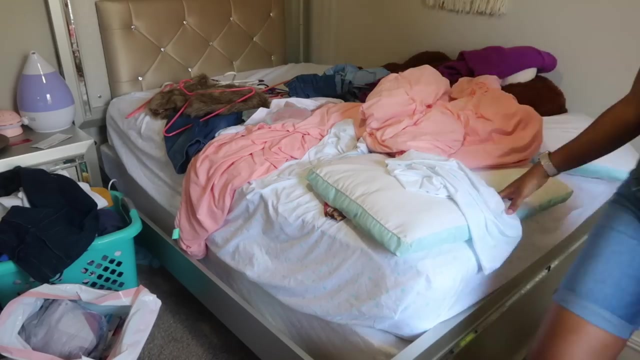 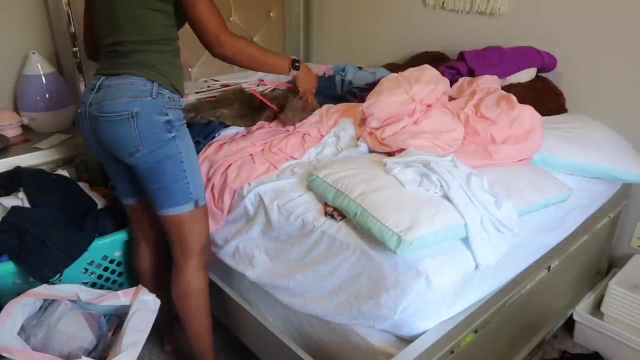 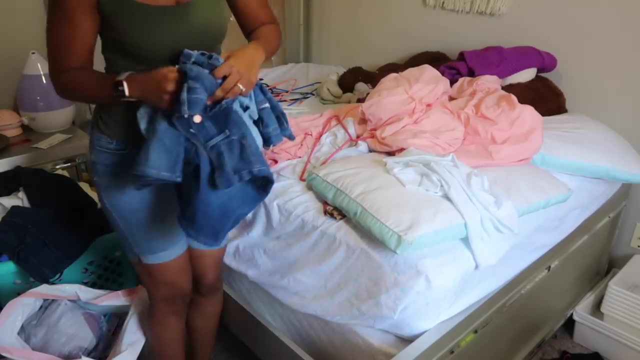 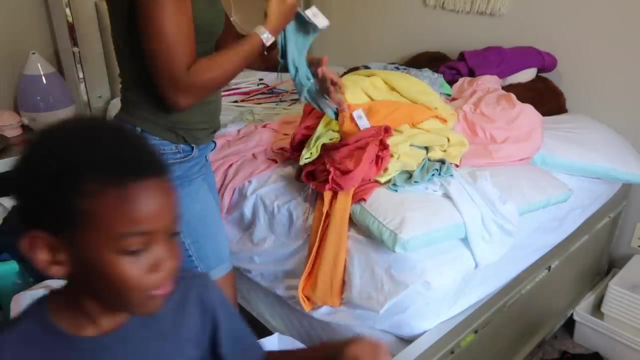 now this little dress I just can't get rid of. it was her birthday party dress from her fifth birthday, and that little fur vest is so cute- something she got, I think, for her fifth birthday, but it was so cute on her- and those two things I can't. I can't get rid of them. so that's why those always stay. and here are some of the new. 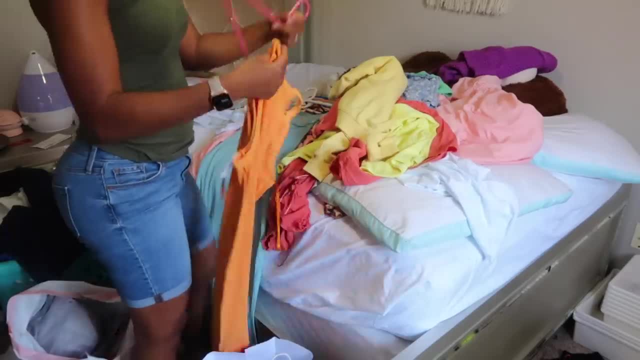 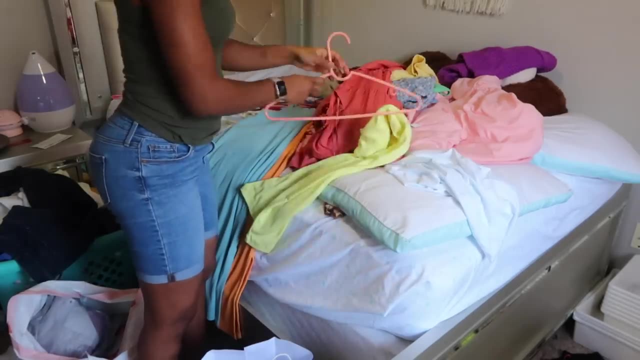 items that I purchased her, that I'm just going to hang up, and no, I don't always wash the clothes before we get them. sometimes she changes her mind, sometimes I change my mind and I want to take things back, even after I hang them up. I've done it plenty of times. I've done it many times. I've. 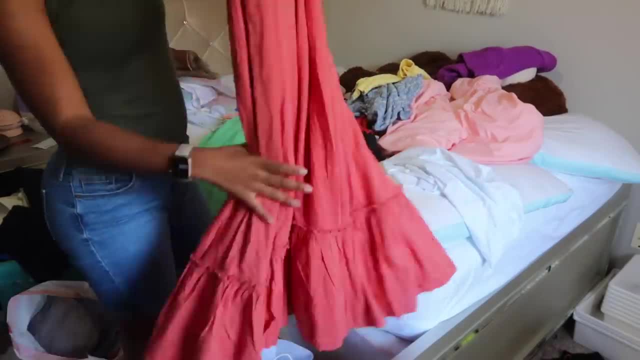 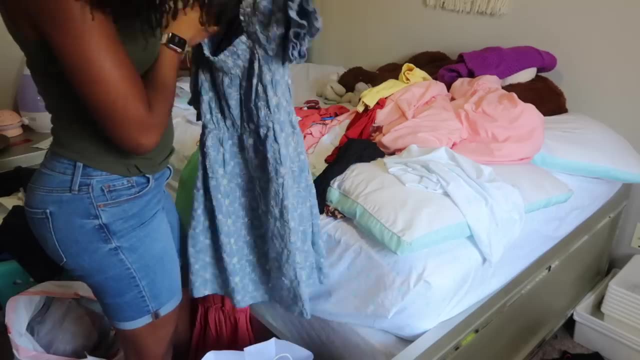 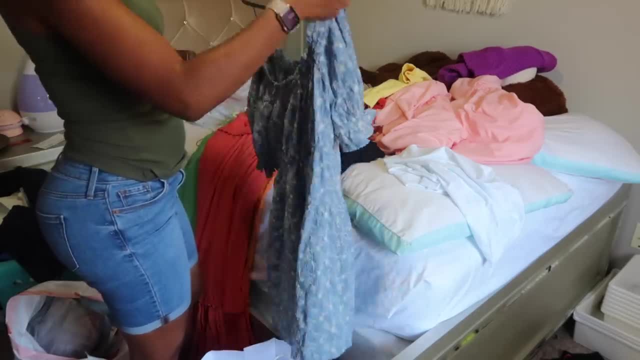 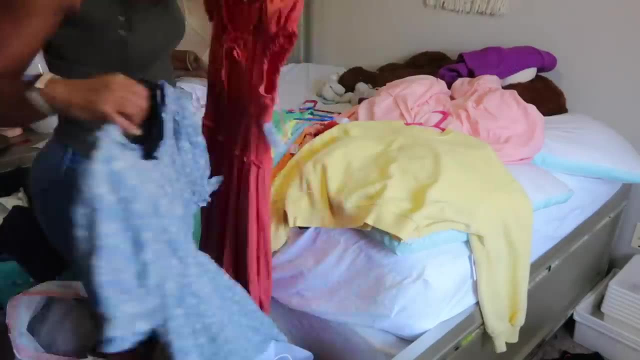 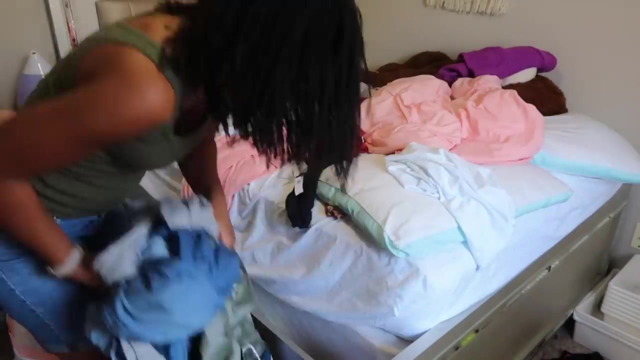 spreading color on this, what we do. and, by the way, the new dress is from anmingjiecom, so go take a look at that for yourself. next, pantyhose spillover, let's go. so these new blow fish are basically a duo winner, and items were for from Old Navy, these things that I just pulled out the bag. 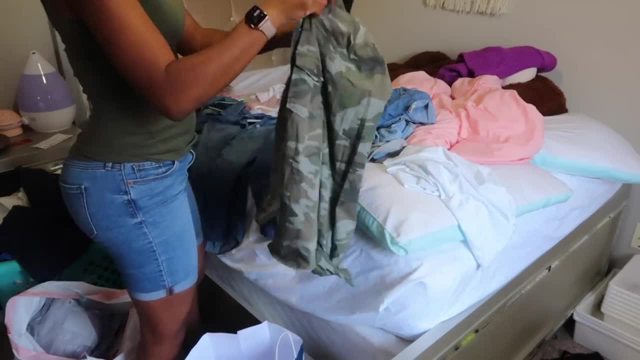 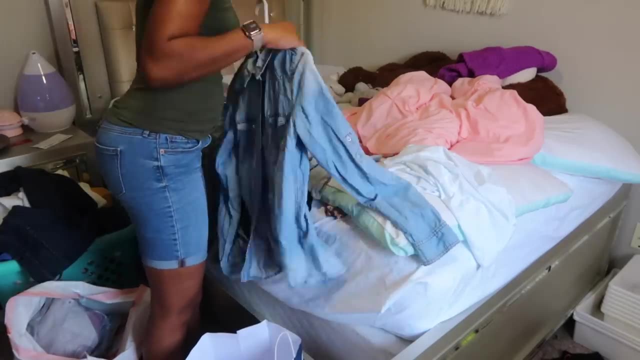 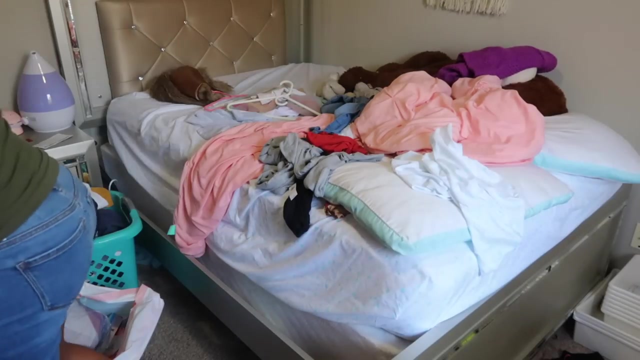 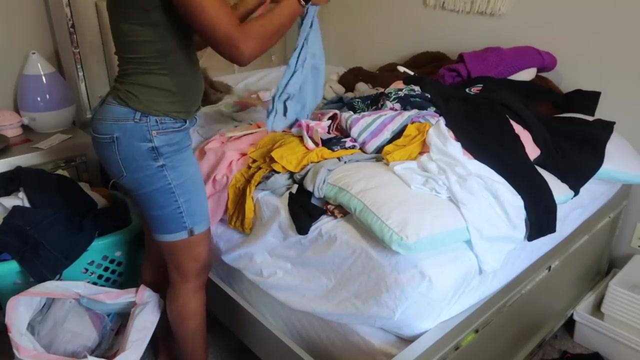 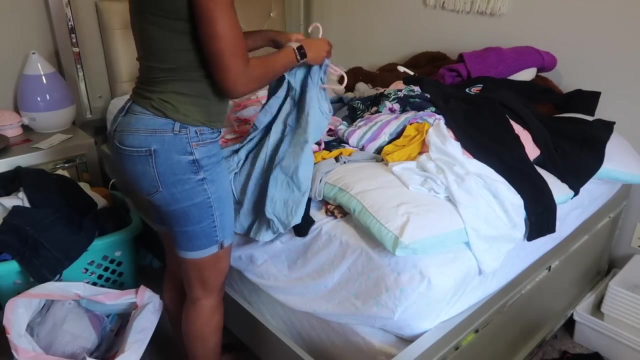 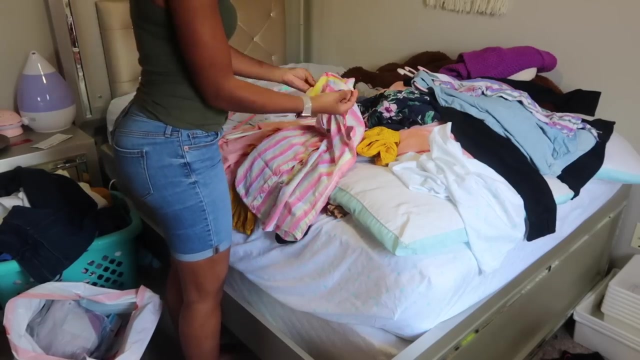 right now aren't new. those are just hand-me-downs from my closet. those are things that no longer fit me and she wanted to keep, so I gave them to her. it was at this moment I realized I have to buy her some adult hangers. she has a. 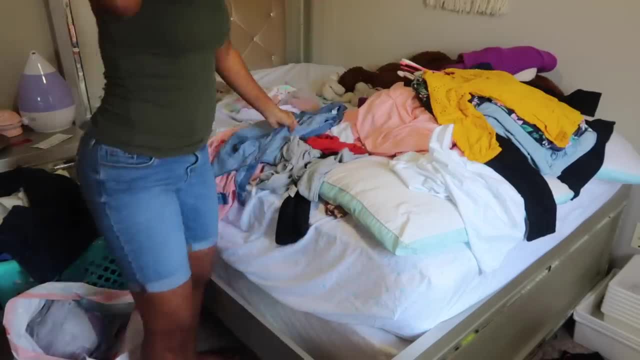 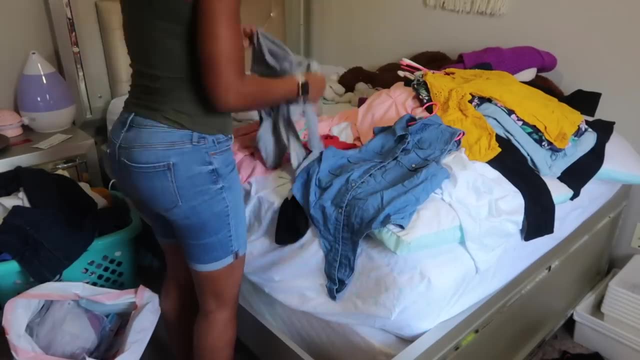 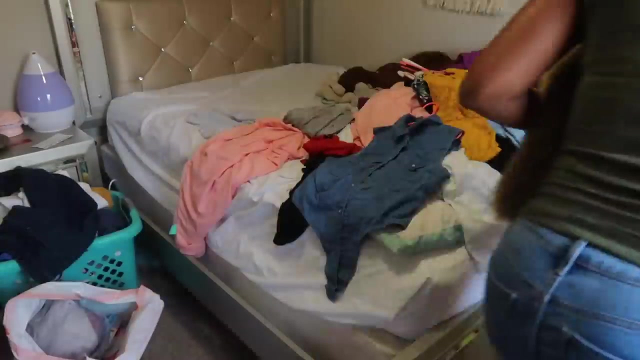 few of our old ones, but most of her hangers are baby hangers and her adult sized clothes just don't fit properly on baby hangers anymore, which I'll show you in a second- Kind of made me feel some type of way. but she's a growing girl and she's growing up beautifully, So it's okay. 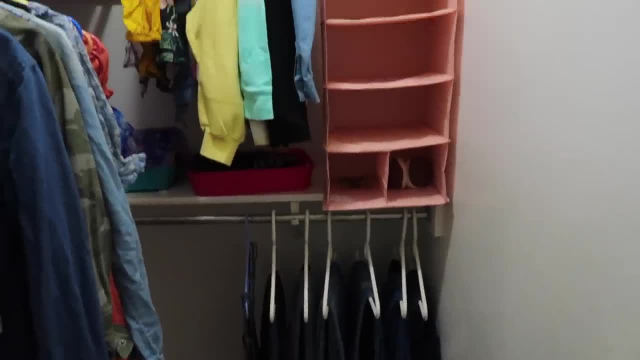 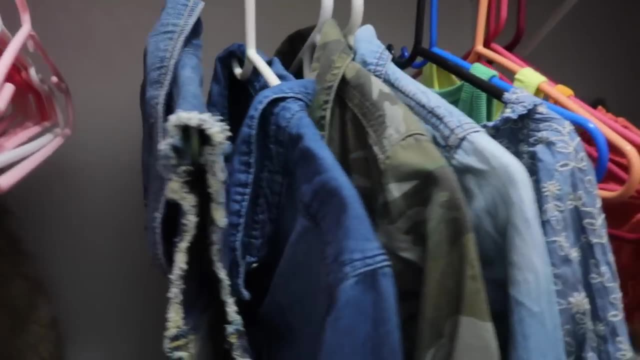 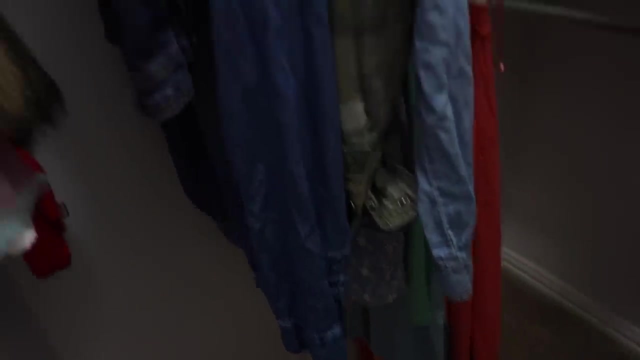 So here is an after shot of her closet completely cleaned out and now everything that is hung up in her closet is Clothing that she can actually wear or she does actually wear. so it's nice and easy for her to Look through her items, see what she Wants to wear in the morning and get dressed. 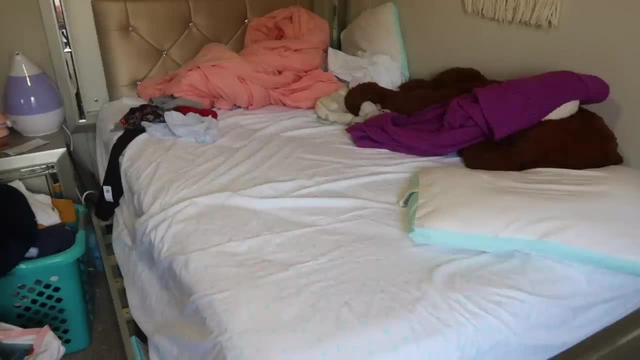 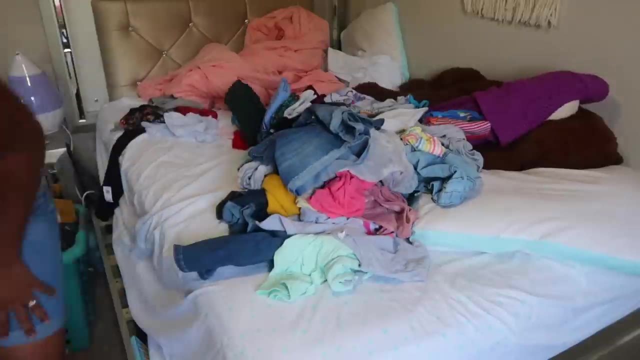 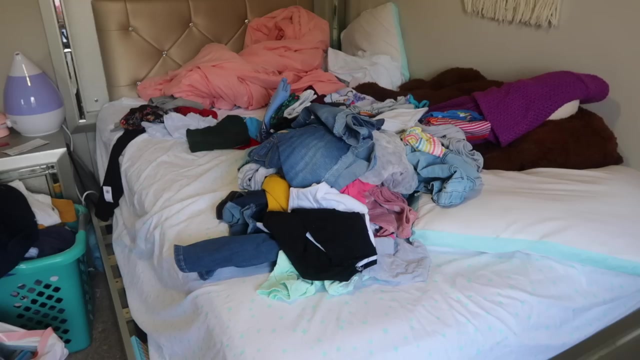 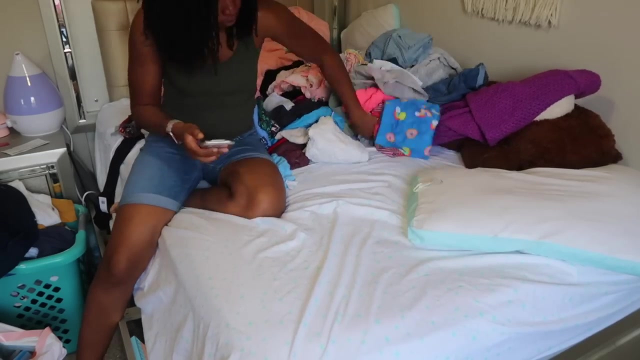 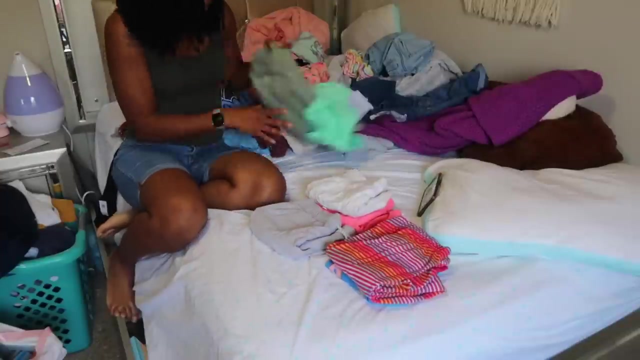 But, as you guys already know, that was only a quarter of the battle, So now I am going to tackle all the clothes that belong in her dresser. About anyone, Hope, ring the stone. Doing what you do, doing what you do. just keep on Doing what you do. Doing what you like, doing what you like to do. 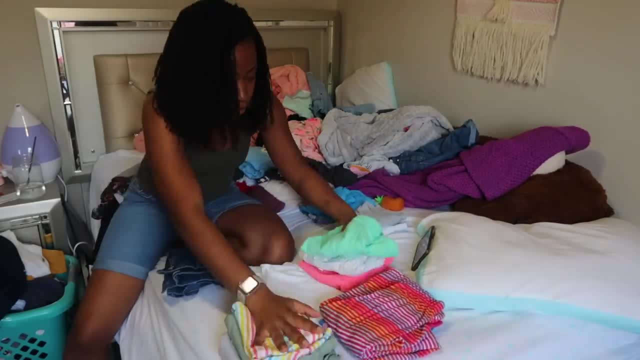 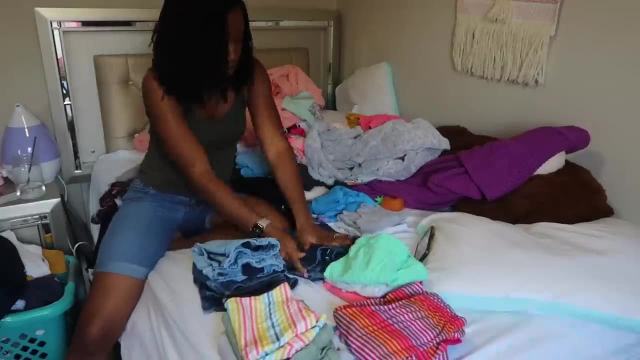 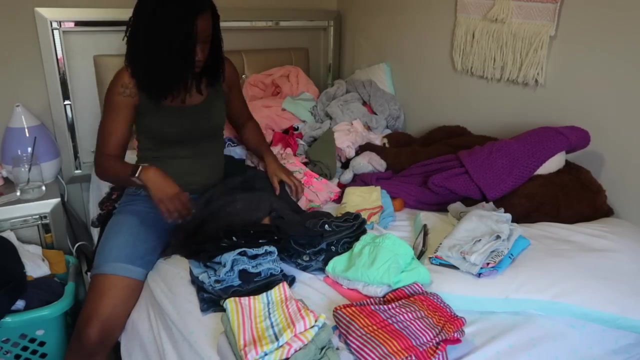 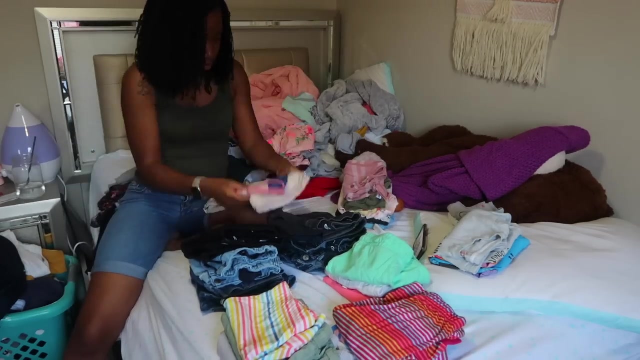 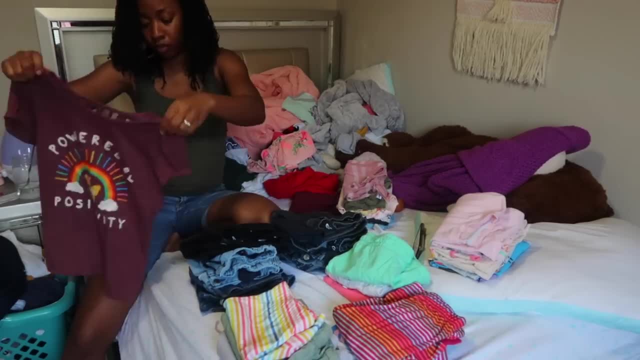 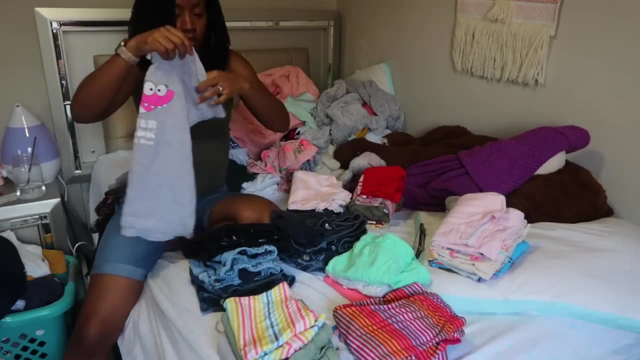 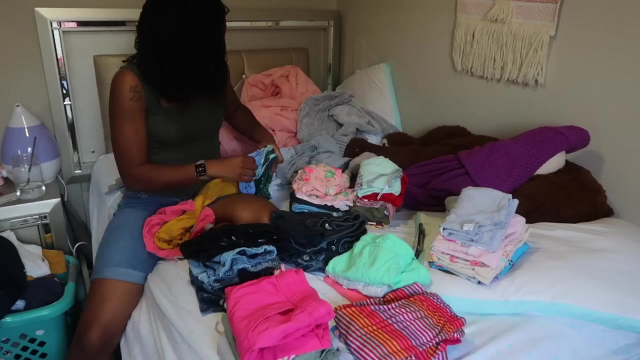 everyone always keep falling in love again. the fuck's wrong with them. i don't understand. maybe it will pass by. someone. save me for a pass out. i'm too lonely to be done. i'm gonna drink at this page. yeah. why am i the only one who's left in the rain with nobody to hold on to? 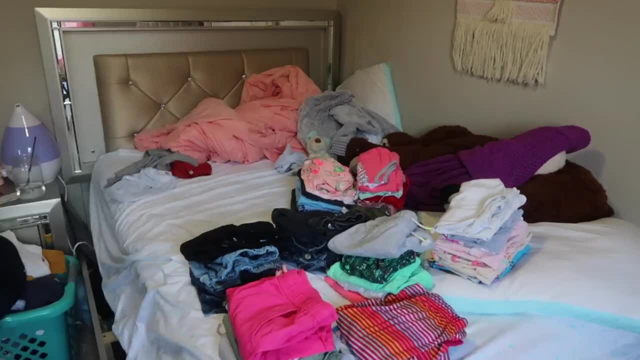 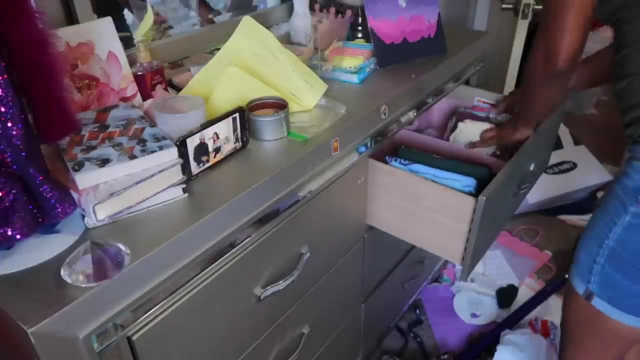 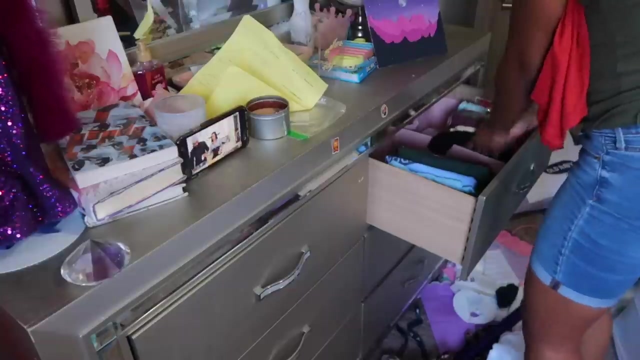 why am i the only one who's feeling this pain? so now that everything is folded, i am going to put them back in the drawers, and i'm putting them back in the same categories as i had them before, and we're going to have a conversation about that again. so the first drawer that i am working on now: 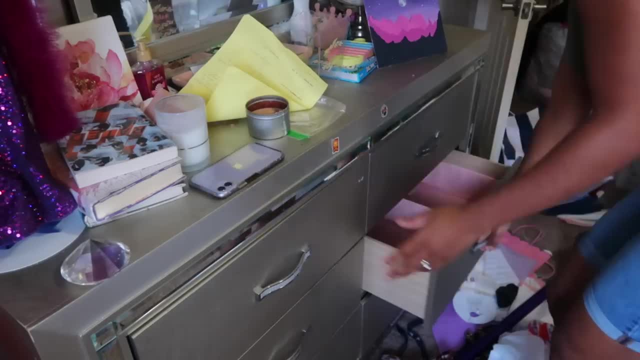 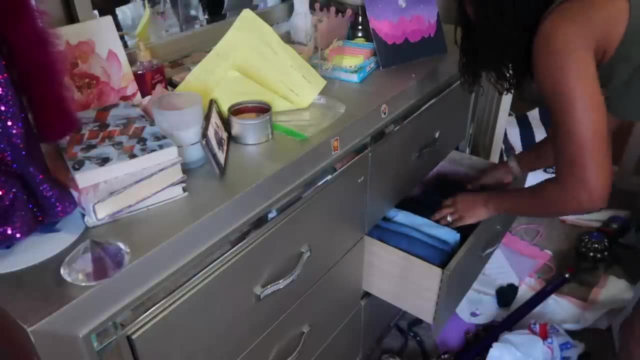 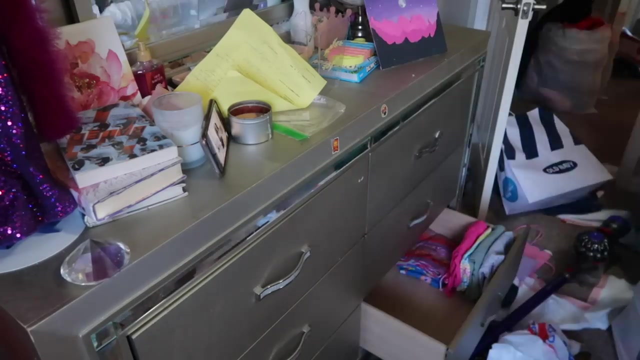 that is for all of her t-shirts and just short sleeve shirts. second drawers are is for bottom, so all of her shorts go in there. you- some of you are probably watching- like why are you telling us y'all, you need to tell her? i'm telling everybody so y'all could help her remember. so if she watched this, it'll help her. 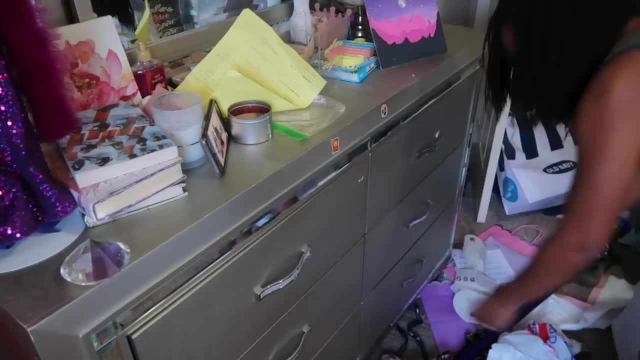 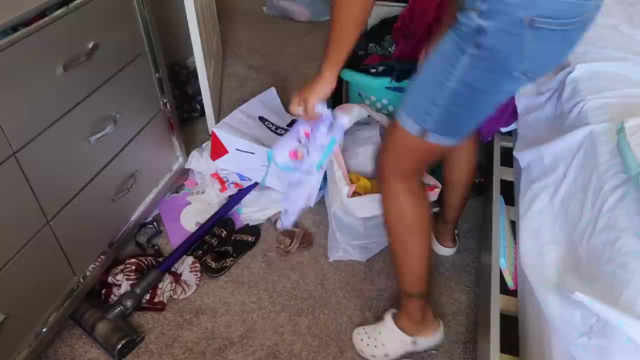 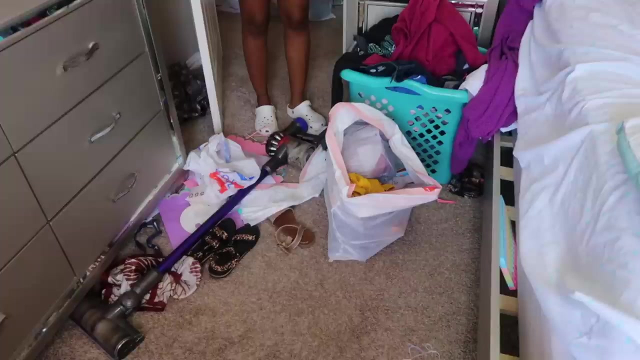 remember, because i'm sick of telling her- i was watching siobhan from siobhan melody tv. i was watching her latest videos when she was cleaning out her twin girls room and she made a video of her twin girls room and she made a statement that you know. 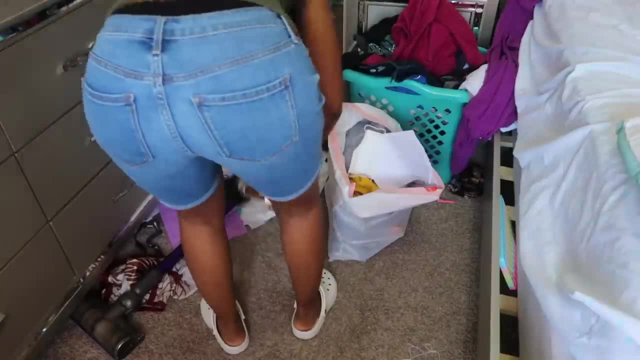 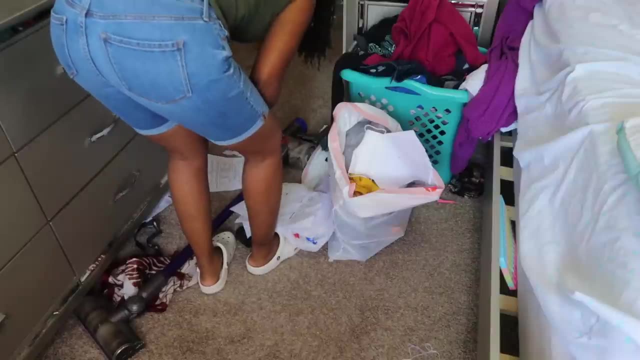 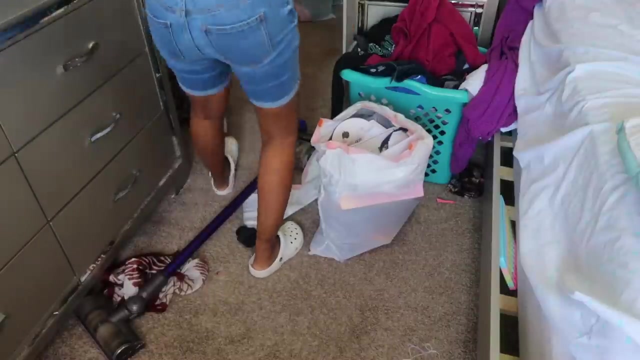 i definitely felt her. she was basically saying that it is time for all these kids to start pulling their weight. you know, we teach them, we talk to them, we're trying to train them, but you know, kids are who they are and i do think that they have this false assumption that because their moms, 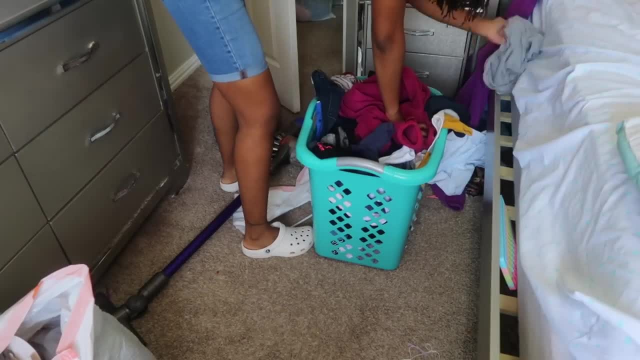 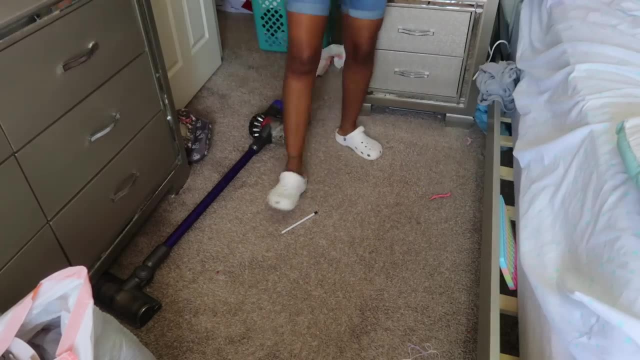 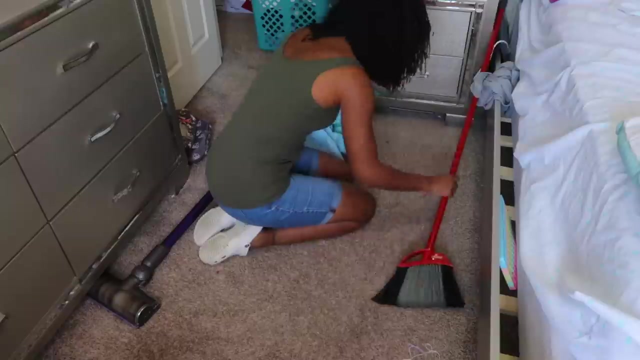 make cleaning videos for youtube that we're okay with this mess because it's content, but, like siobhan said said, there is always something to do in the house. I do not need you to help me create mess. I need you to maintain your own living spaces and help me maintain our home. So we had to have that. 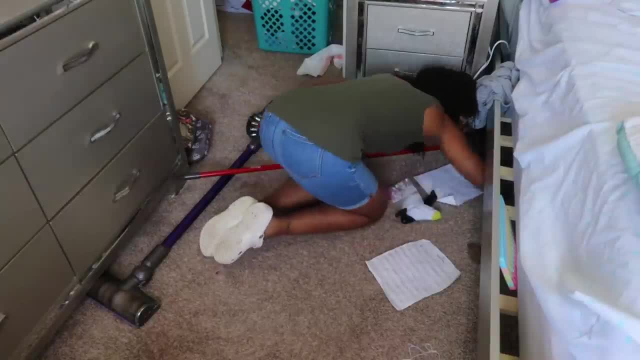 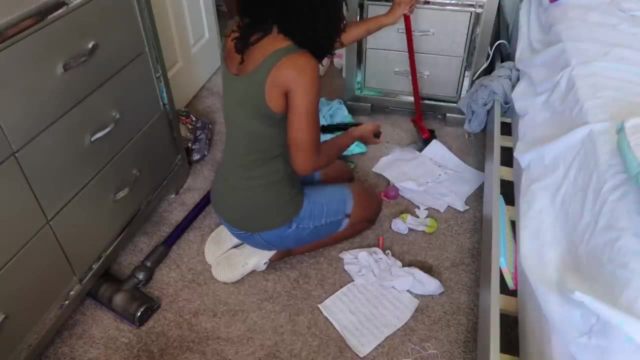 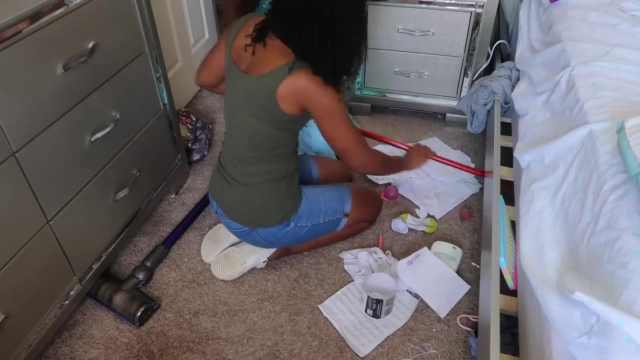 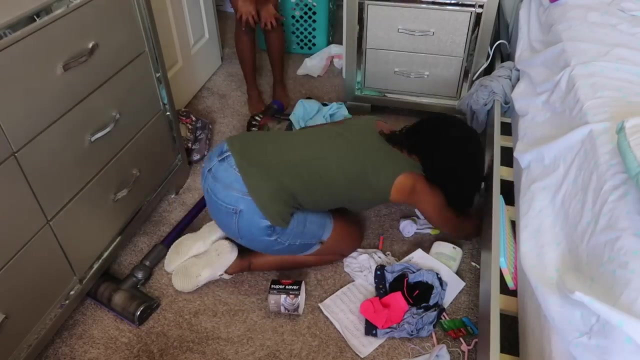 conversation at my house as well. So this girl had so much stuff under her bed, My little broom hack wasn't working quite well and I refused to climb up under her bed to get all of that stuff out. So I sent her under the bed to get. 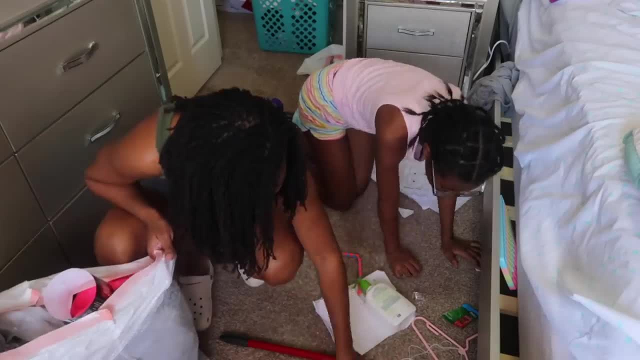 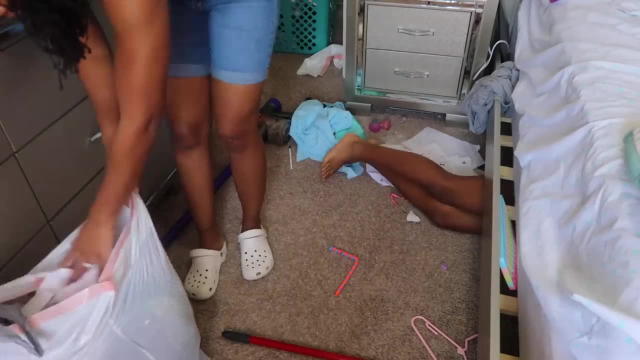 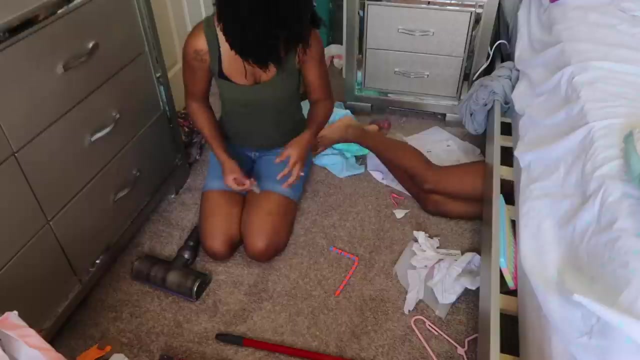 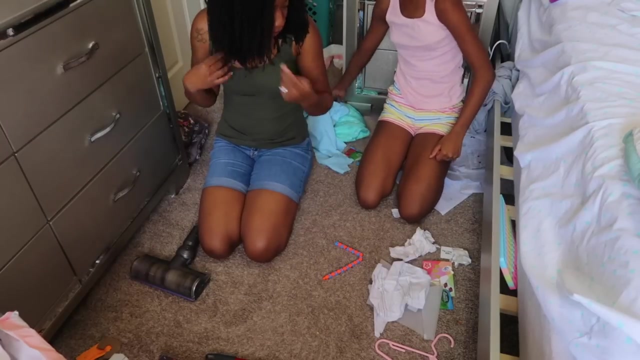 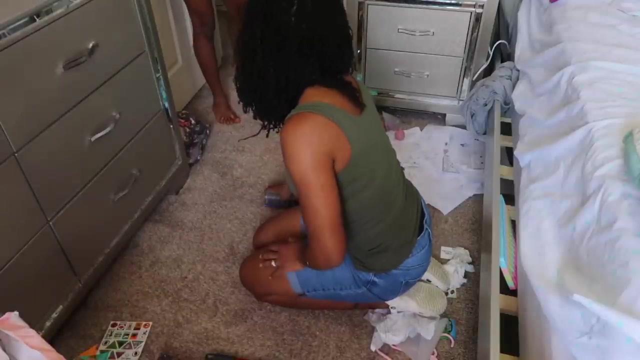 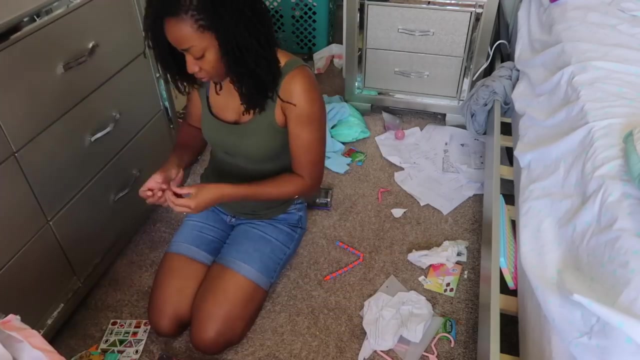 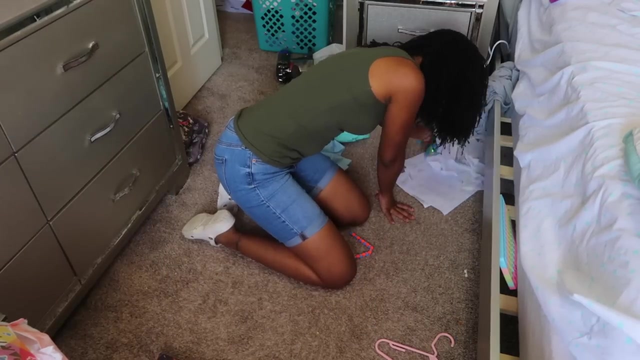 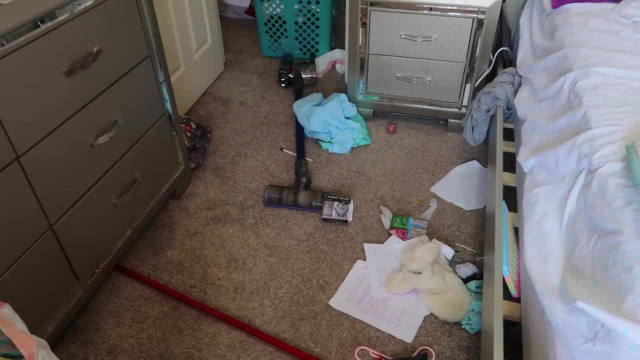 the rest of the junk out. Right now I'm standing in a corner. I see you from across the room. It's kind of crowded here, but I know you see me too. Everybody's singing, oh, Everybody's singing. oh, I don't know what it is about you. It must be in the way you move. Just say you want me to. We got. 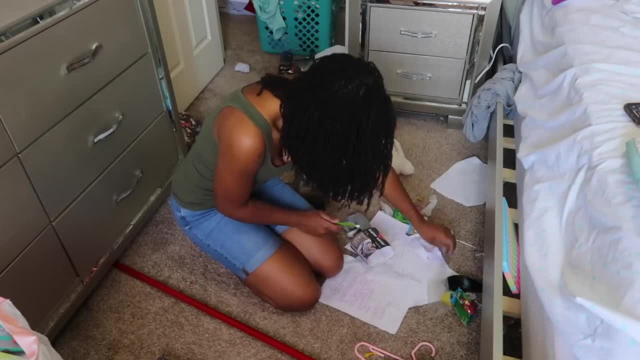 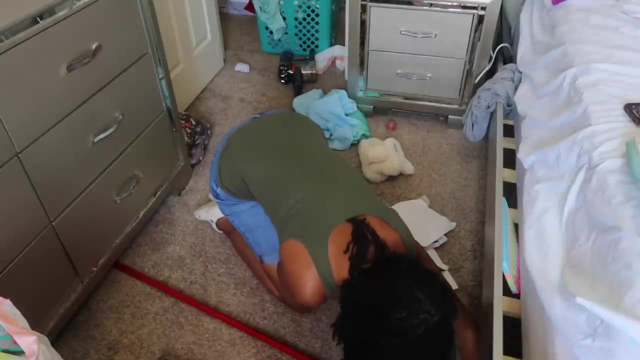 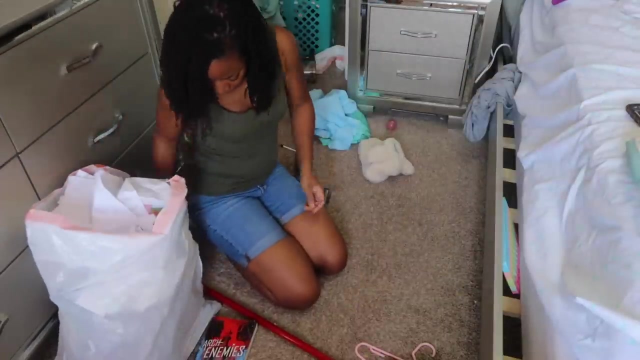 nothing to lose. You're looking so old. You're looking so old. Now I'm moving closer to you And it's getting dark in this room. Tell me what you want to do, Baby. let me love you. Let me love you. 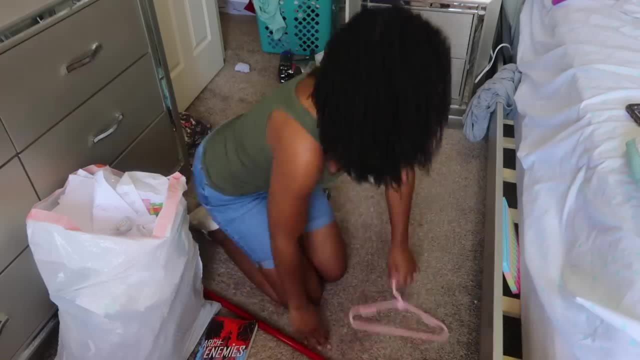 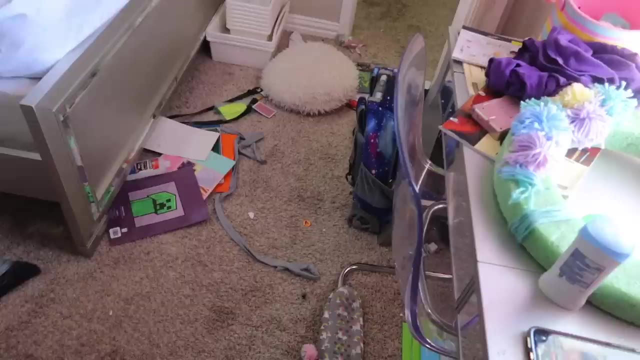 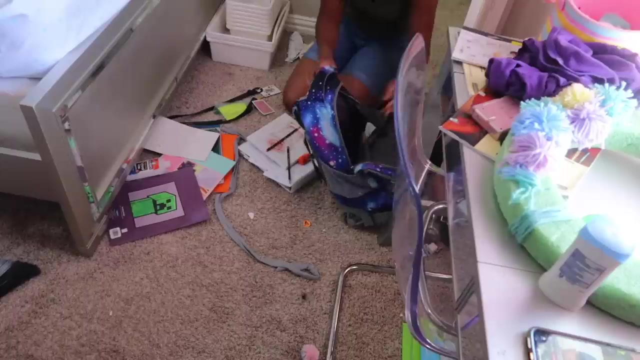 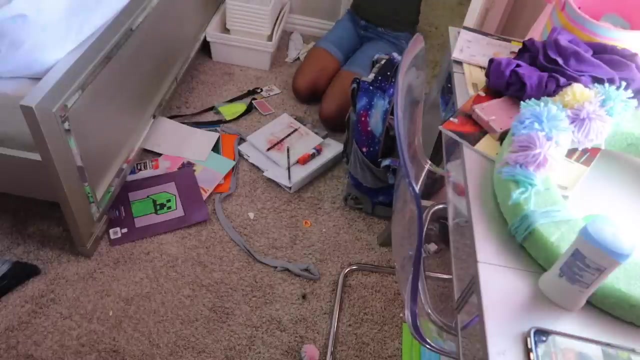 Let me love you, Baby, let me love you, Let me love you, Let me love. Let me love, Baby, let me love you. Just say the word and we can leave this place. I'll take you anywhere you want, As long as we're. 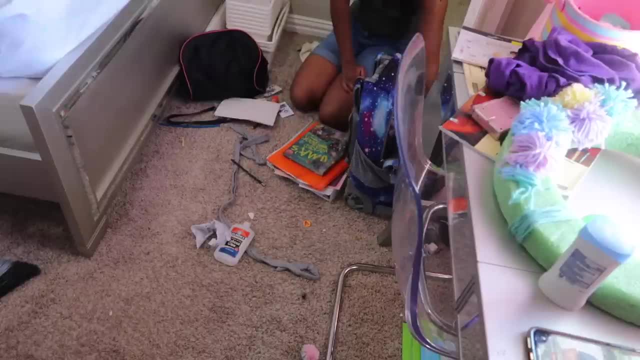 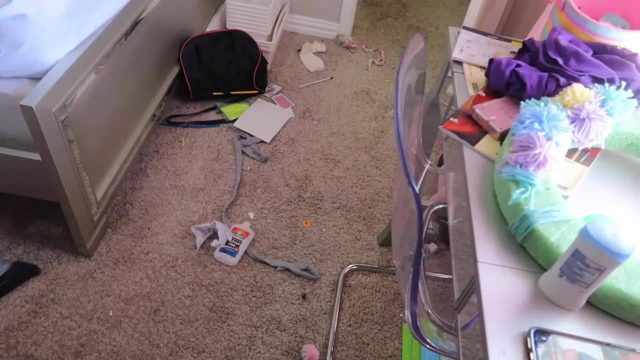 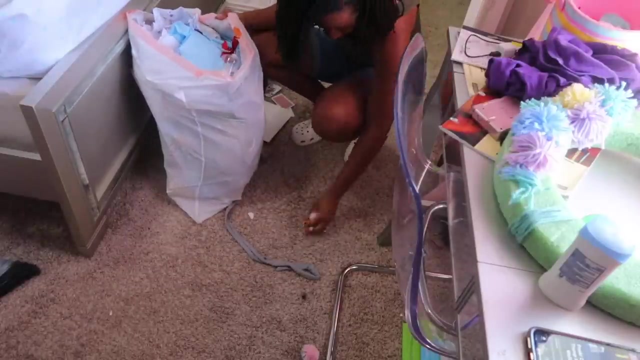 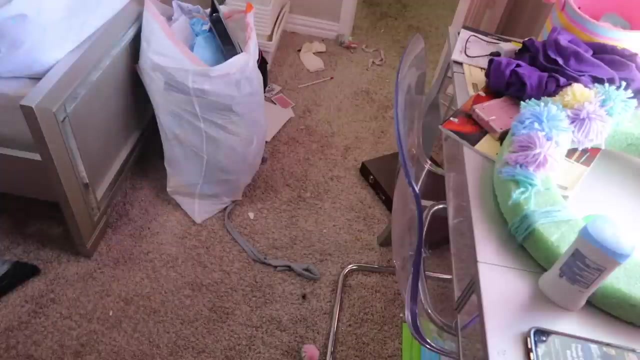 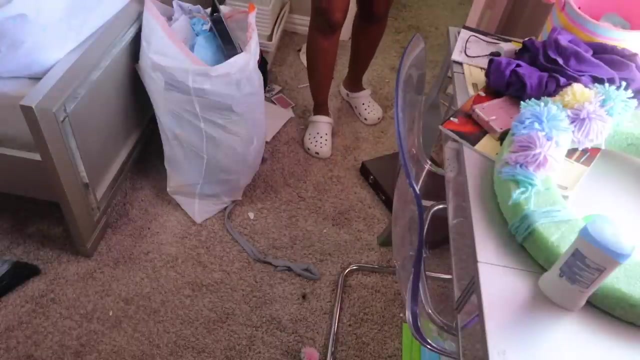 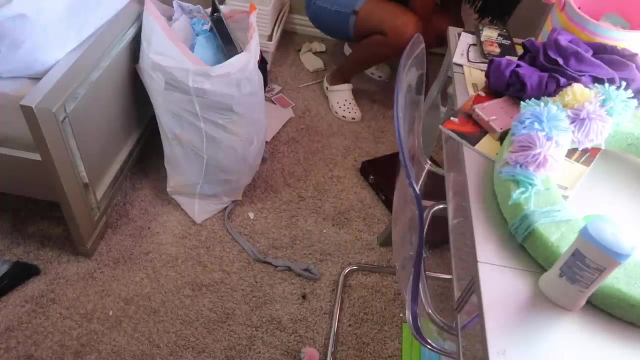 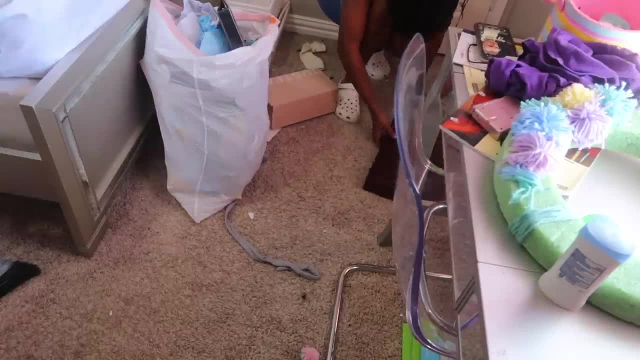 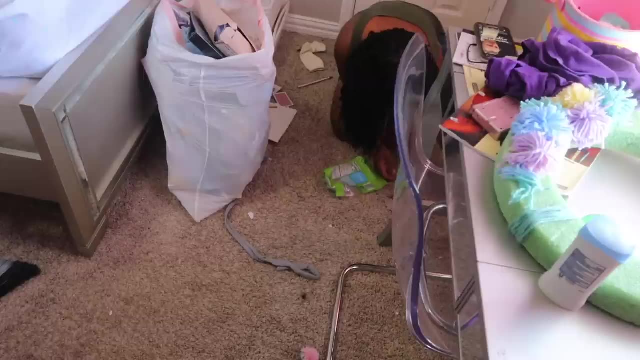 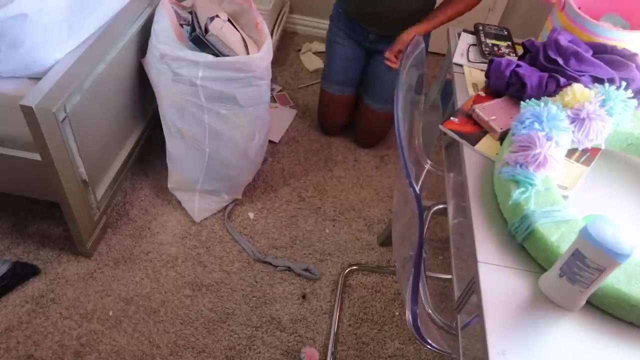 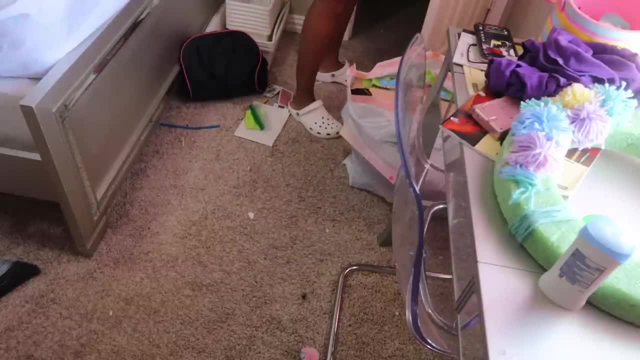 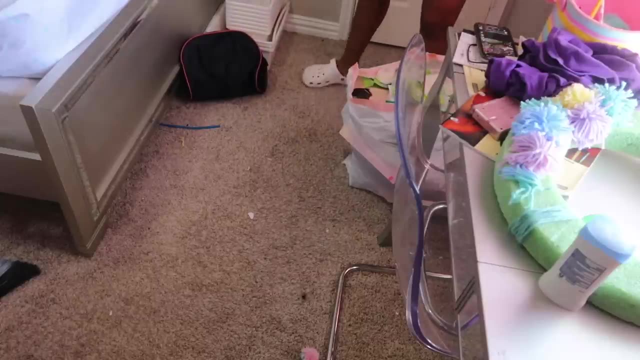 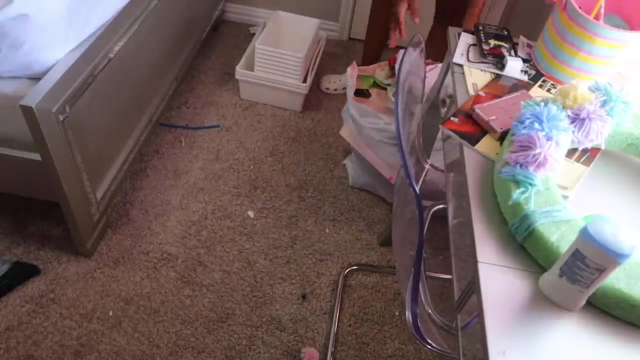 It's almost like you make me fly When I look at you smile. I don't know how, but it feels like I'm drunk on you. it feels like i'm drunk on you. it feels like i'm drunk on you. so this was definitely a lot of work, to say the least. um, so i've been gently reminding her. 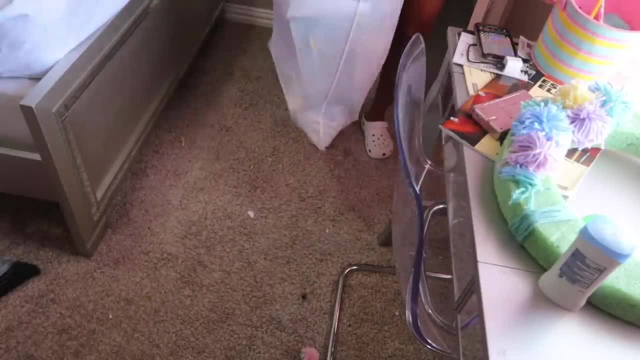 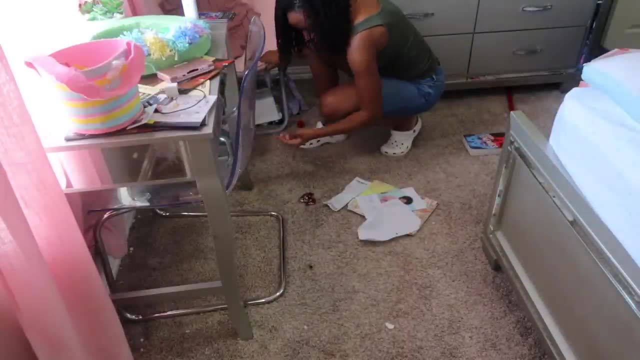 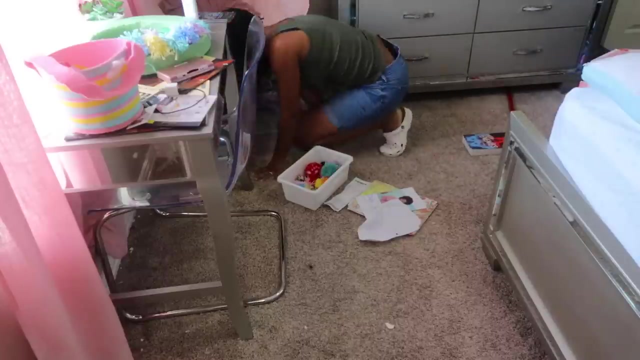 daily or every other day to just kind of keep up after her stuff so that it doesn't get out of control like this again. i am trying to monitor what she brings in her room, especially with that backpack. i'm about to ban the backpack from coming upstairs because i feel like she packs. 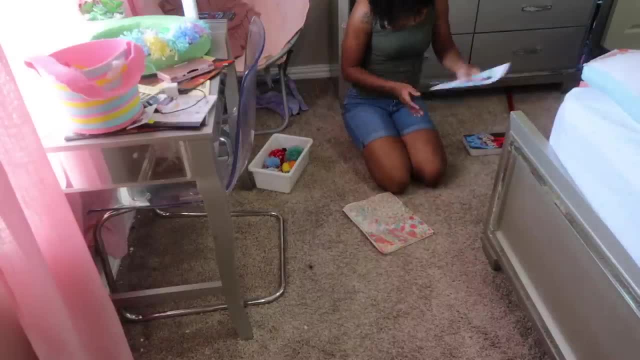 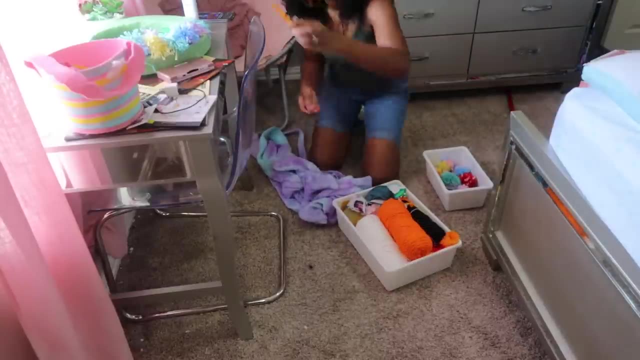 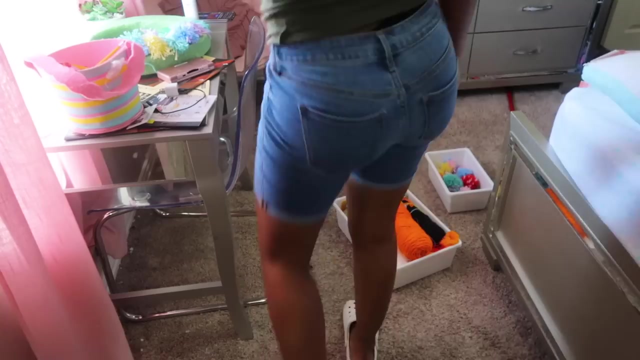 things in her backpack and then brings it upstairs and unpacks it in her room, because i just don't understand where a lot of these knickknacks come from. but i've been monitoring it because i do not like to spend an entire day, or what feels like an entire day, cleaning one room in my house. 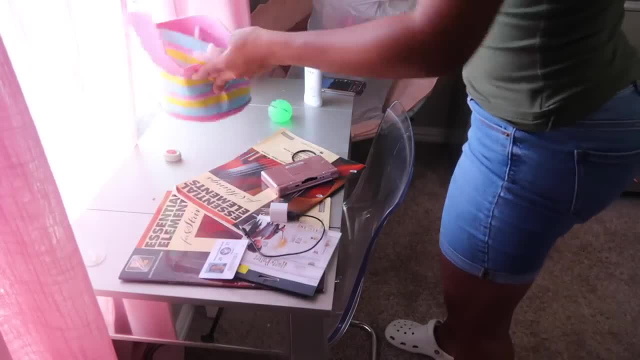 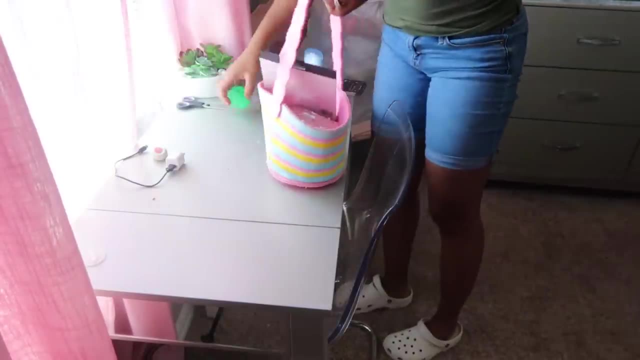 i need some time on my own to figure out what i want, and i just want to put another little disclaimer out there. i know i don't have to- the people who support me are probably going to tell me i don't have to- but sometimes i just don't want to deal with certain type of comments. i am not. 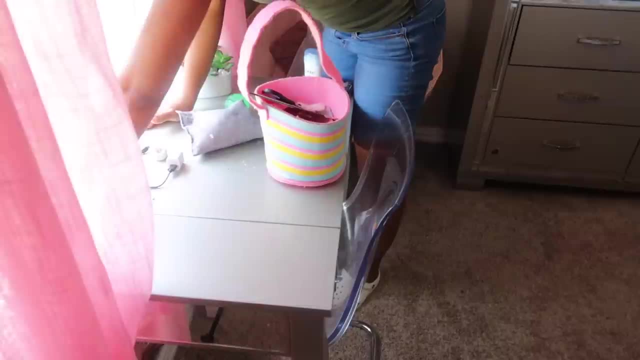 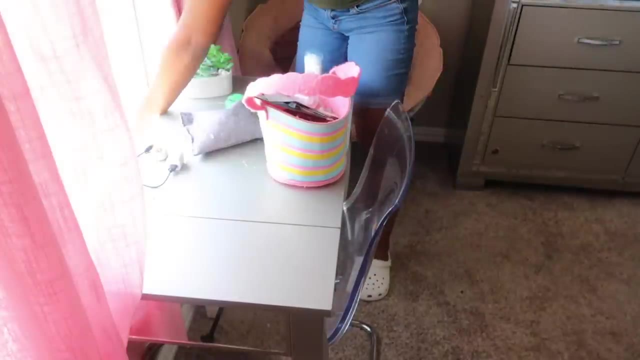 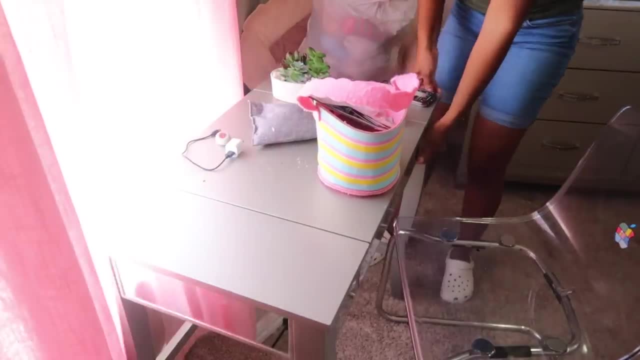 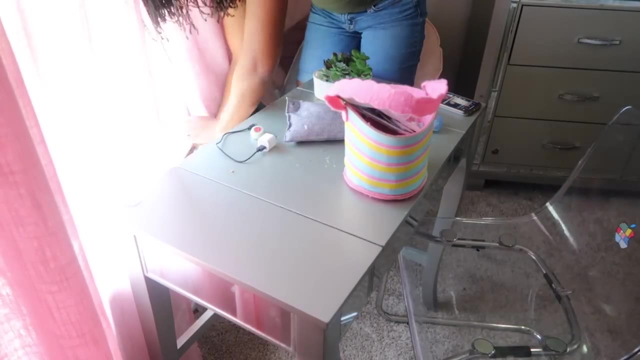 she plays the viola and violin. she spends many hours a week in orchestra and doing concerts. she's a very busy kid so i know she's doing the best she can. it's still frustrating sometimes because i feel like she can do a little bit of a better job than she is. but again, i'm not soliciting. 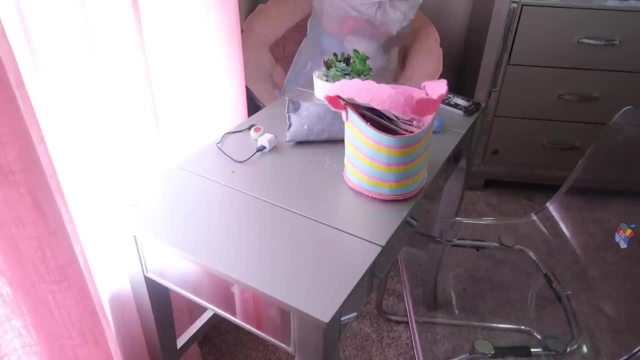 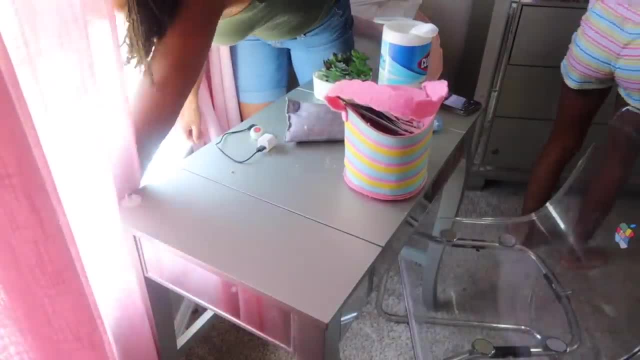 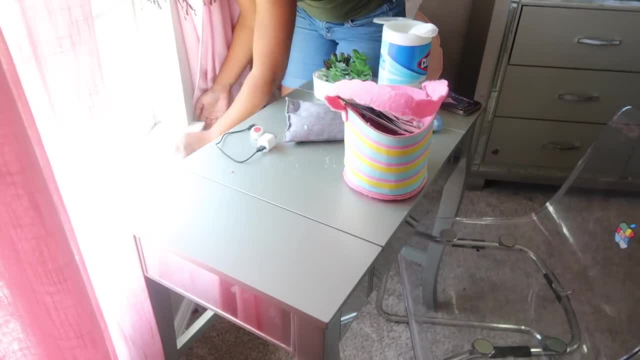 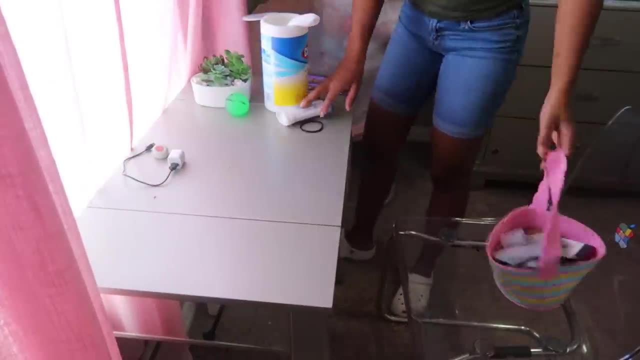 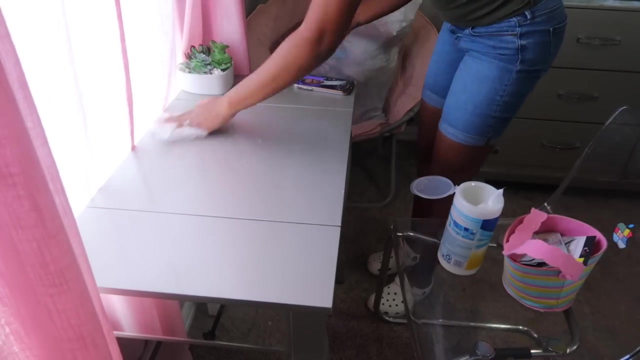 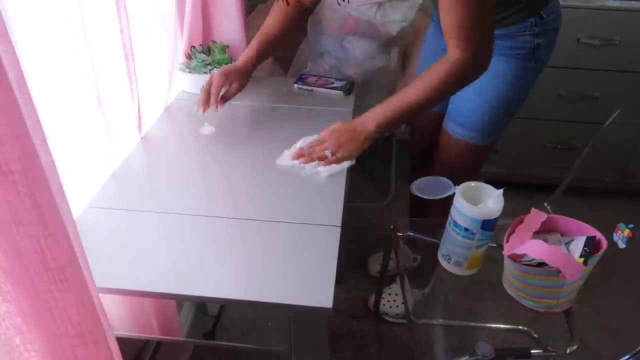 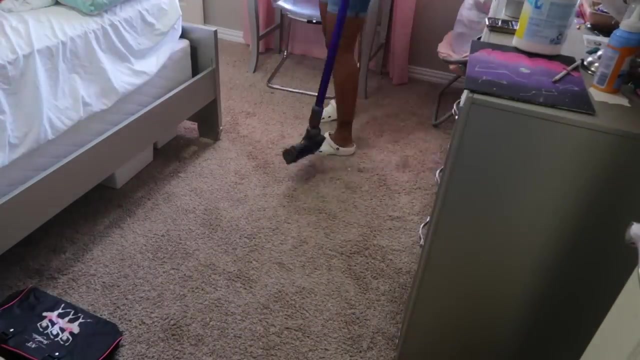 it's just that i'm an adult and i know how to clean up my mess- how to clean up my mess- and she's still learning that. so, and she's still learning that, so it's okay. I need some time on my own To figure out what I want. 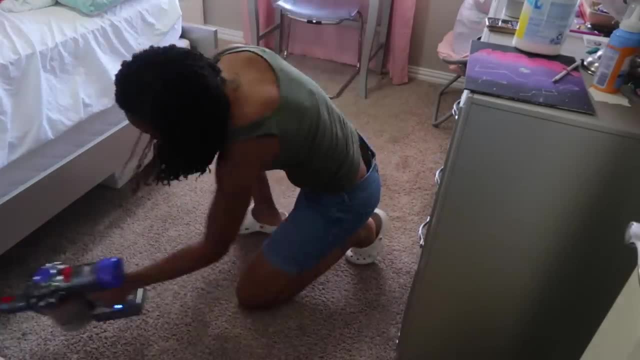 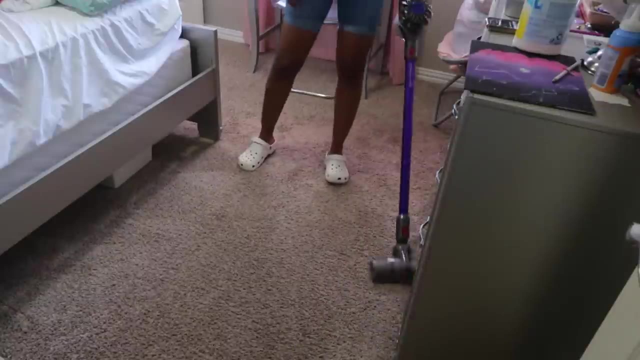 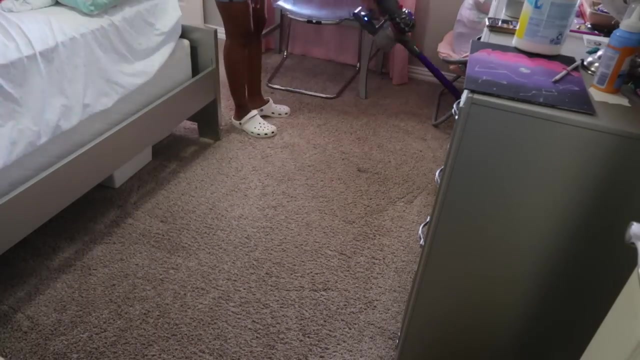 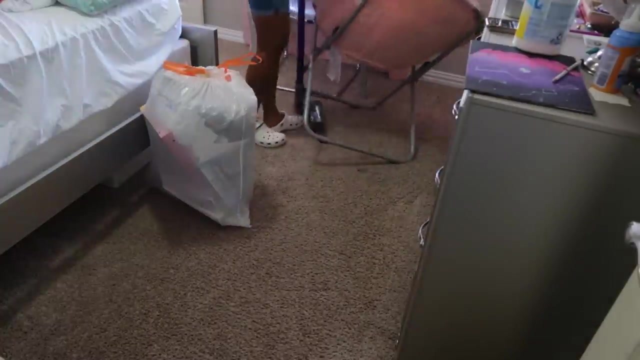 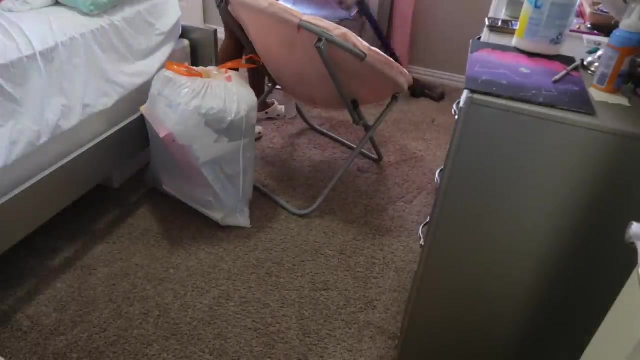 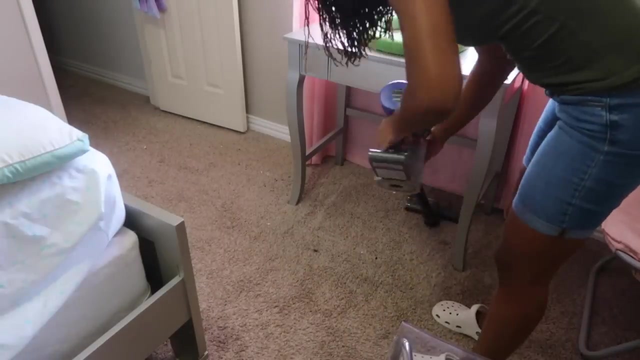 Cause. baby right now- I don't know- Feels like I'm riding solo. You got me thinking about All of the problems in us. I know it's sad, but we both know Maybe it's time that I let you. I know it's time that I let you. 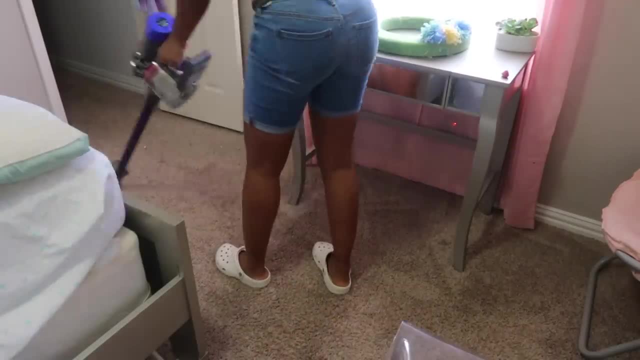 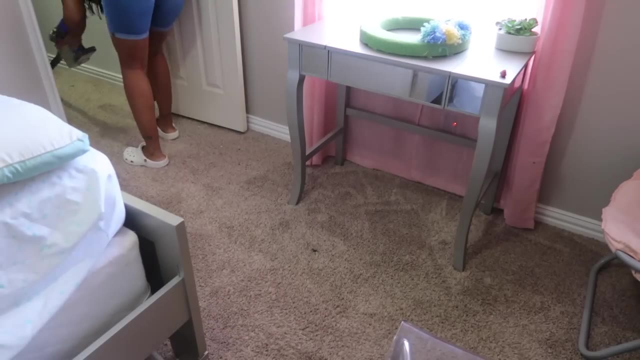 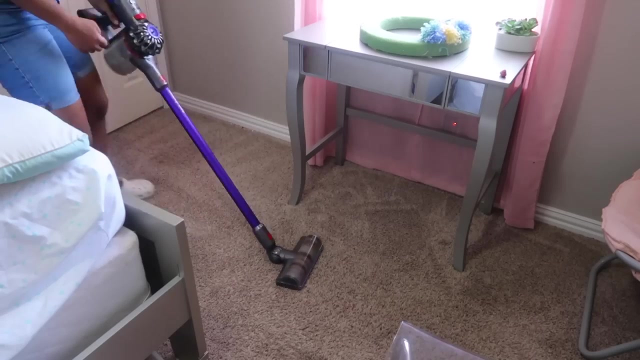 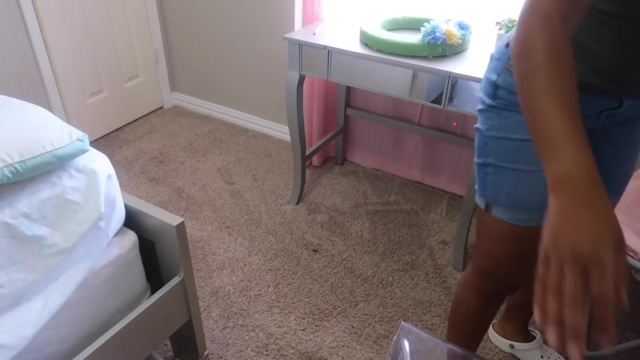 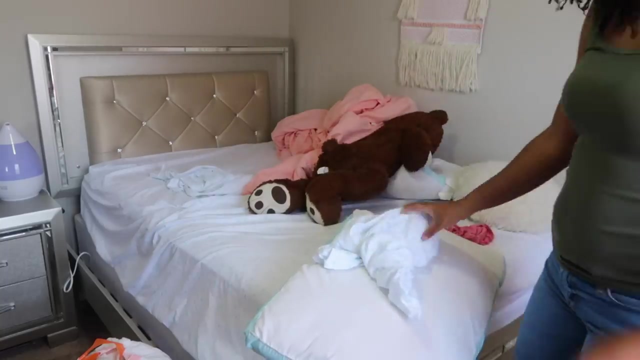 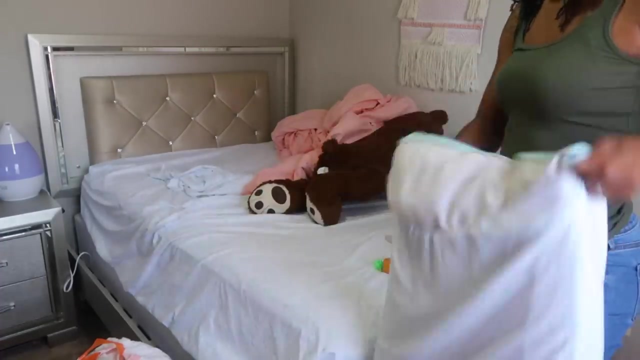 Every night I'm going on the grid Texting back. I want you Hit you up. I'm on the other side. I miss you, Miss you. Take you off. I can't Me. wait is drunk, Can't? no? keep it low key. Got me drugged. your pheromones hit the roof. Follow your taste. It's really a bad reception out there Where you heading. Why ain't gravity pulling you in closer to me? I've lost you, But I need you, And you're off my radar now. I've lost you Telling you that I need you. 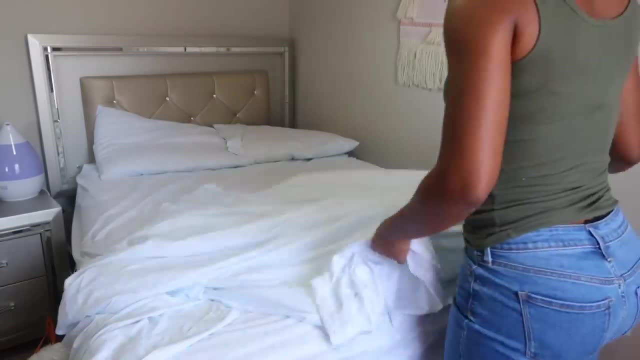 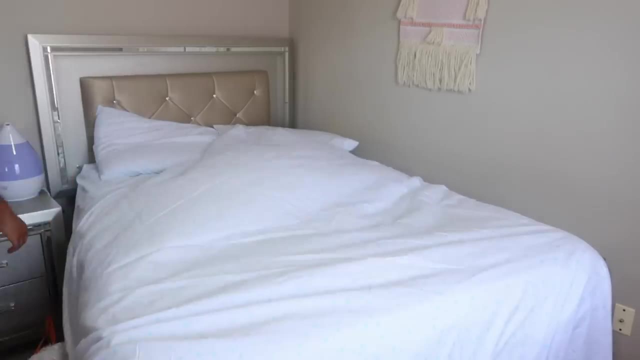 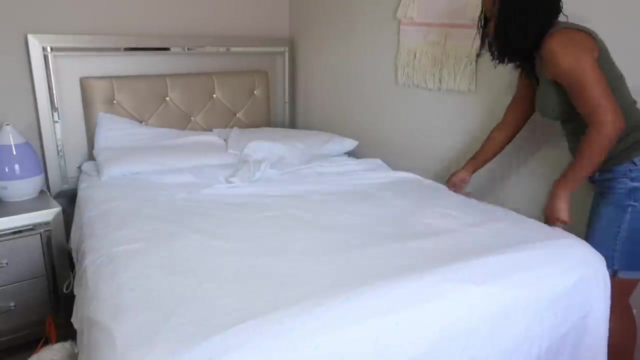 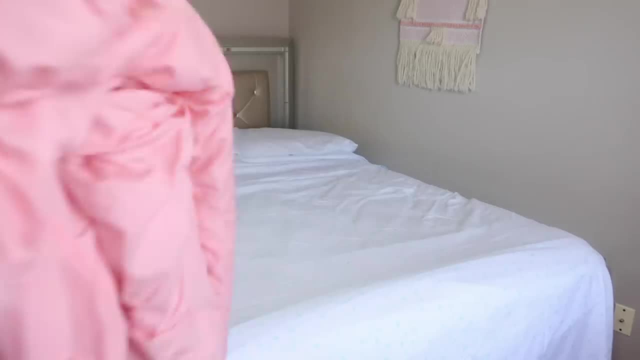 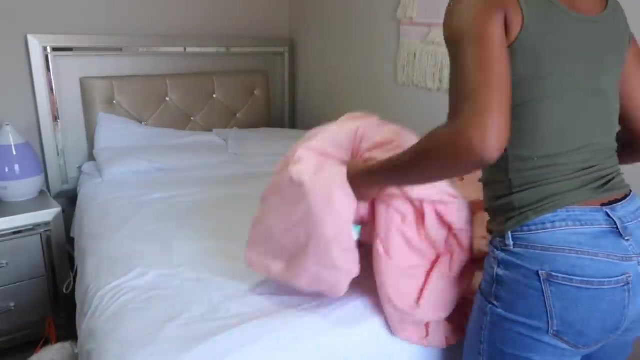 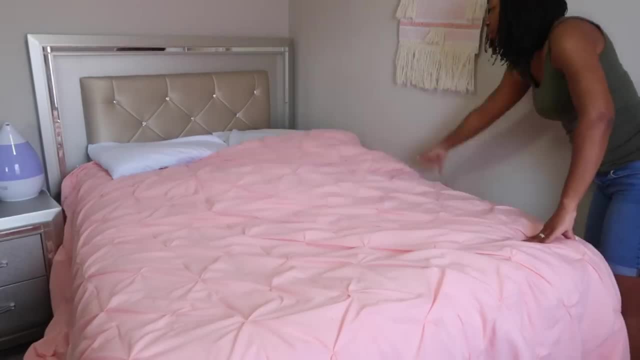 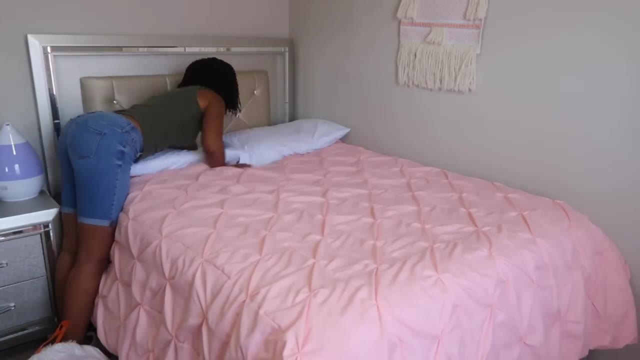 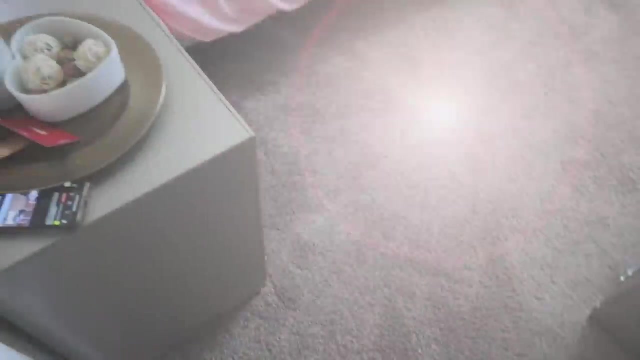 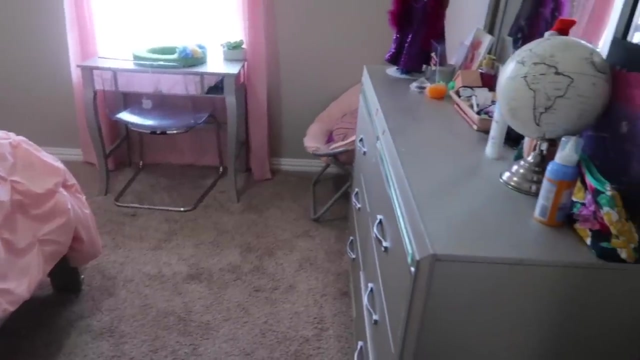 So shameless Can't get enough. I've lost you, But I need you And you're off my radar now I've lost you. I think her bedroom will always be the most satisfying After shot for me, because all that it takes To get this room back in decent shape is insane.